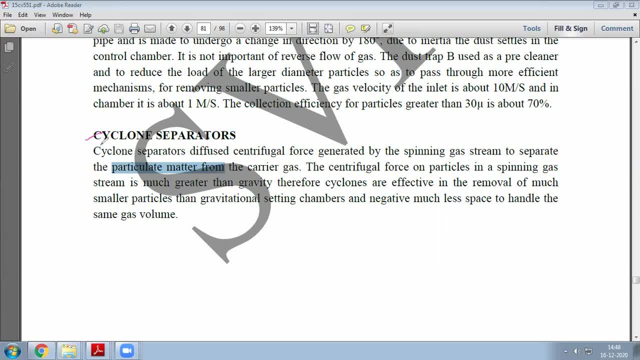 I covered that. it's called cyclone separator, So cyclone separator, I think I covered that. So this used to work by centrifugal force, I think spinning of the gas stream. They used to create one centrifugal force, So that used. 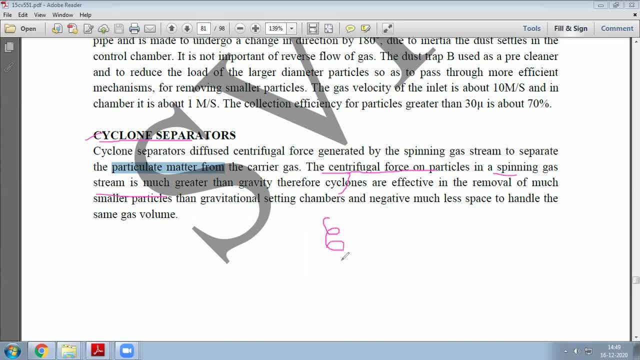 to create some circular flow like this. So, since it was like this the tank, it used to get impacted In the you know here. So that is how it used to get clear. I think it's here. I will show you that. 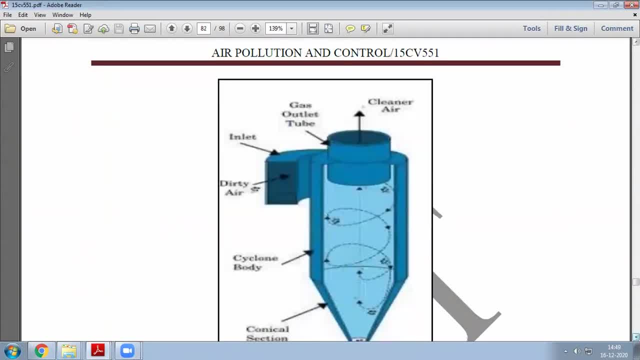 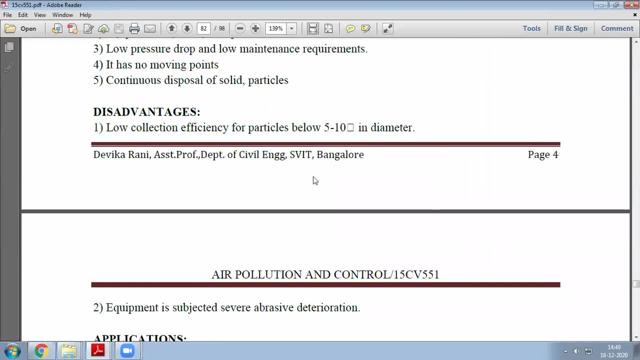 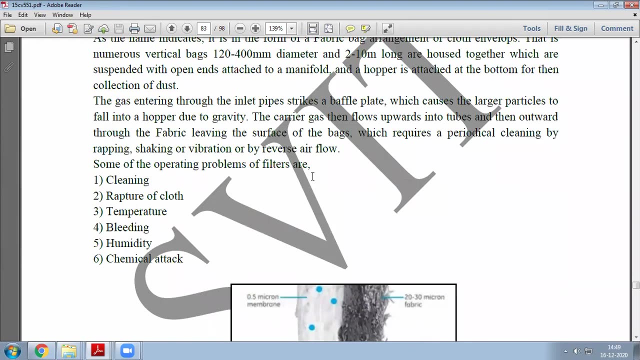 See this, this is how the diagram right. So because of the centrifugal force, it used to remove particulate matter. Now you will see one more method: Fabric filters. This is one more thing. They will install near two industries where you know you have a. 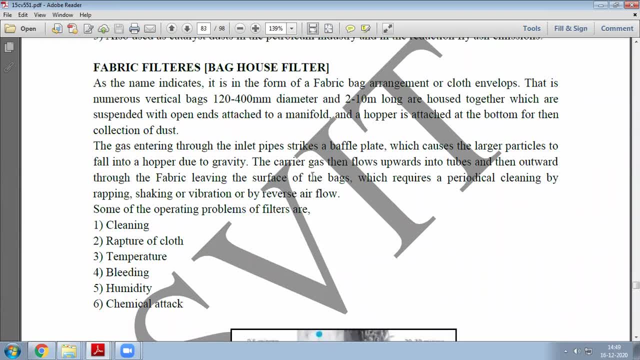 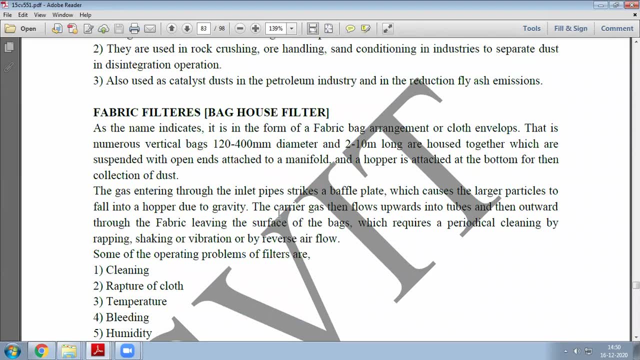 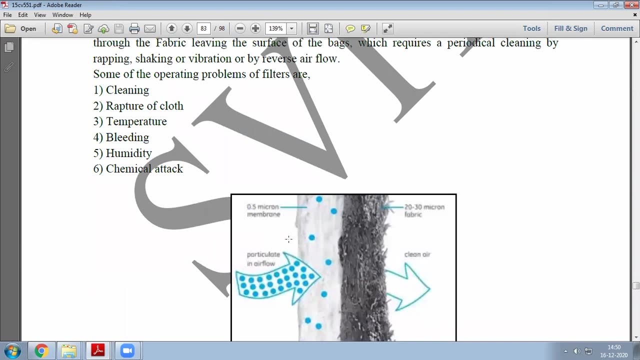 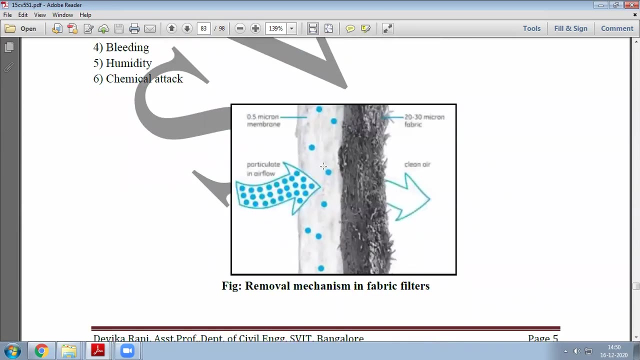 ーム of gasses would be releasing out mainly, or gasses, See here gas, any of the particular guests. like nitrogen outside, something we feel is existing, We can install this or any particulate matter. So actually, if it is releasing in any initial 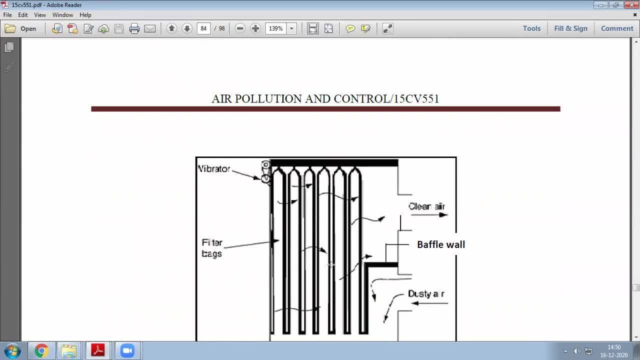 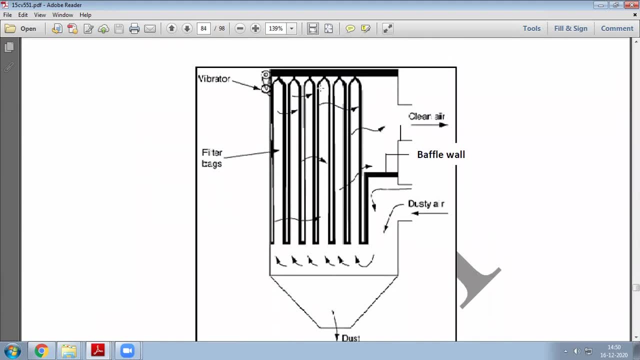 process. they'll install this And those particularly, it will arrest. Okay, So we will see that It will function. so see how it has some- you know- filter bags like this. it will be vibrating. so because of this, the particular will arrest. here is right, it will see. here it is vibrating and clean air will pass to. 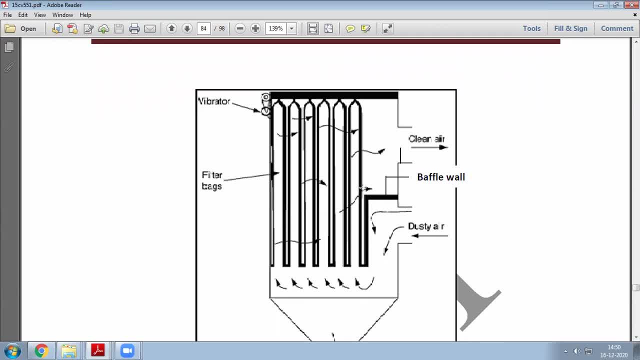 another. so you will see that in how it will function on both as well. also, they will give it here one bottle wall also. they have given here. i think this is the bottle wall. yeah, uh, so this is how it will separate out. i think i covered that. 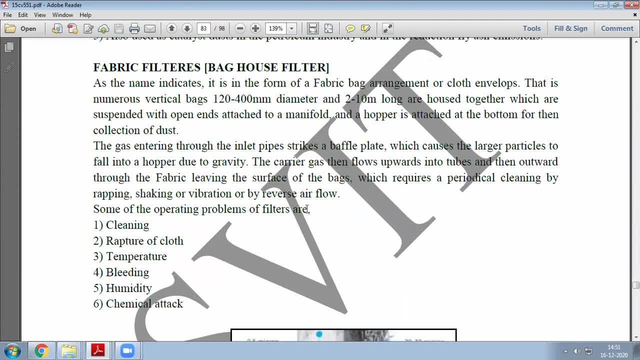 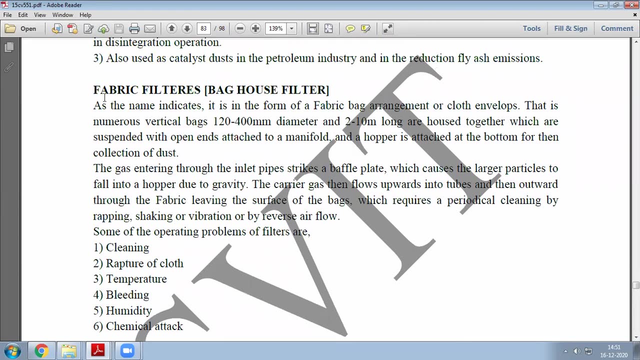 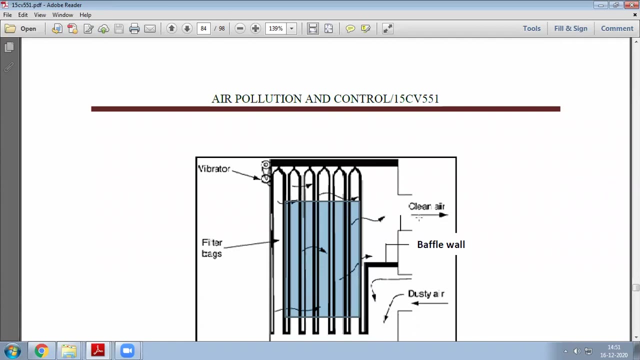 so we will see what the speed up is tells. so one thing you got to know: they will install in any industries where this particular matrix producing. they will install this. so we will see the removal mechanism. okay, so what is this? fabric filter means some fabric material. uh, they have installed it here, right? so that is why the name they have given. just, 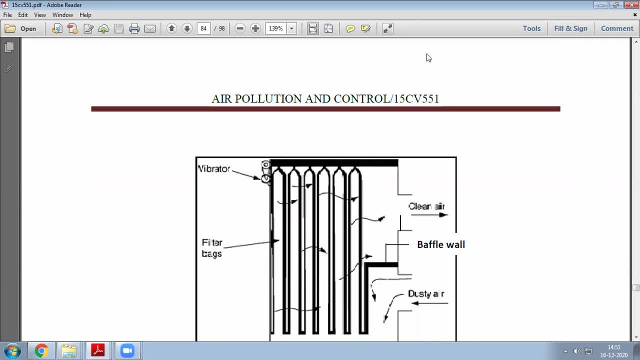 uh, all particles comes out and that will strike here. it will strike like this, okay, and they will be vibrating, so all dirt gas will be removed in the bottom, all the striked particle will go in the bottom and all the clean air. it will go like this, okay. so that is the principle. so i hope you understood. uh, we'll read what the speed? 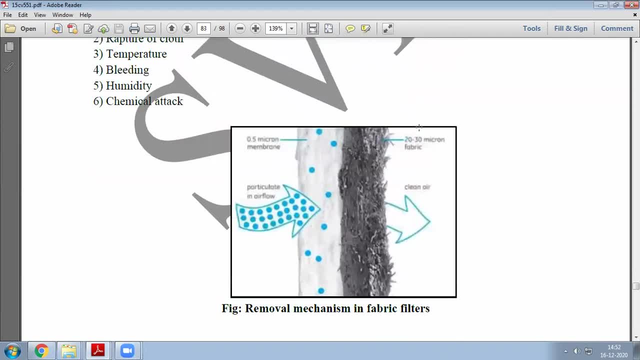 of will say: though okay, see here, so they're given some diameter and all micro. oh, this is nothing but fabric cloth. you can say: one draw cloth any particulate entering no 0.5 micro microbe, so it will arrest here. see here, it's arrested here. 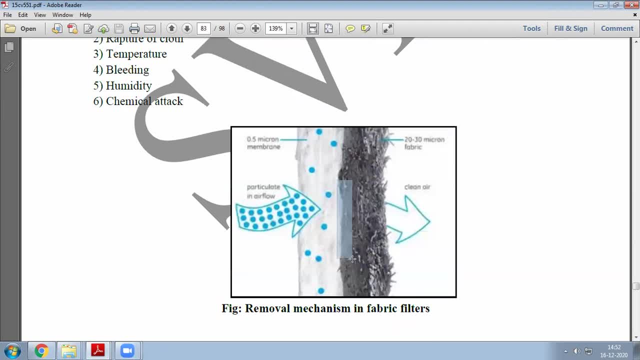 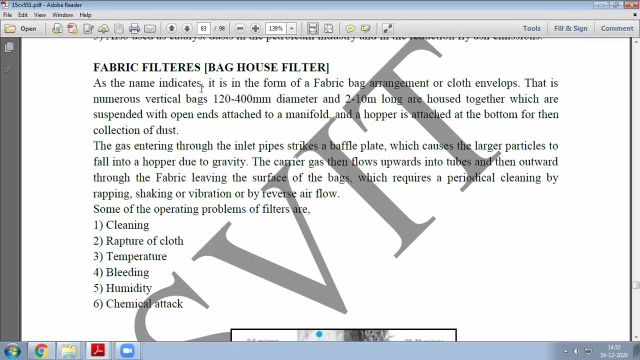 and clean air will pass through one more side, since this will be vibrating now. so all particulate will settle in one section and cleaner will go up. okay, so that is that is how fabric filter functions. okay, so what it is, as the name indicates, it's a. it's a fabric bag. uh. arrangement of cloth envelope. 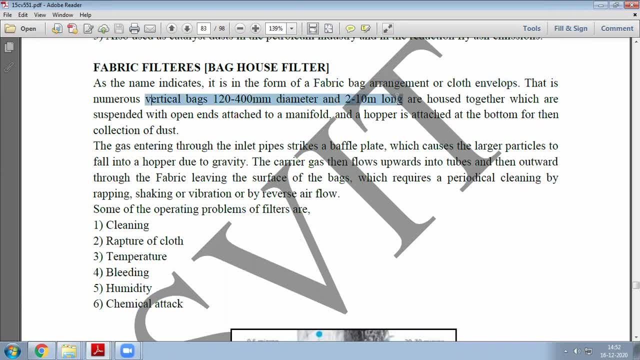 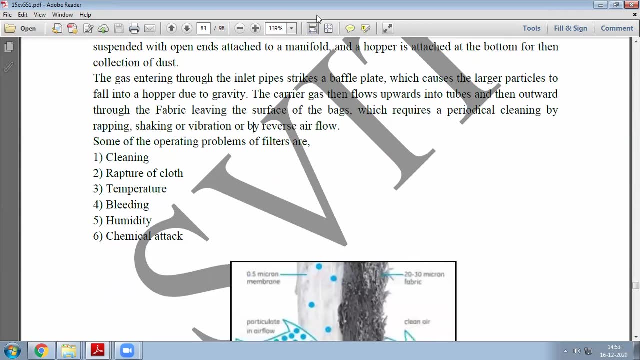 it has a bags of this much of diameter and this much of long. it is suspended, attached in manifold in the bottom hooper is attached so that all you know particulate which is collected it will reach there. so the process they have given in here see, uh, yes. 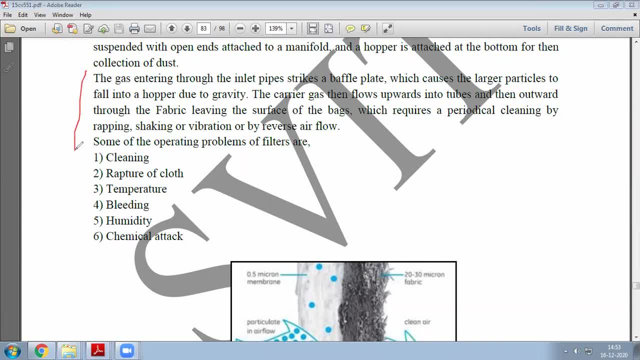 yes, this is all process, they are given. gas entering through inlet pipe strikes the baffle plate, which causes the larger particle to fall into hooper due to gravity. the carrier gas then flows upward into tubes and then outward through fabric, leaving surface of the bags which requires 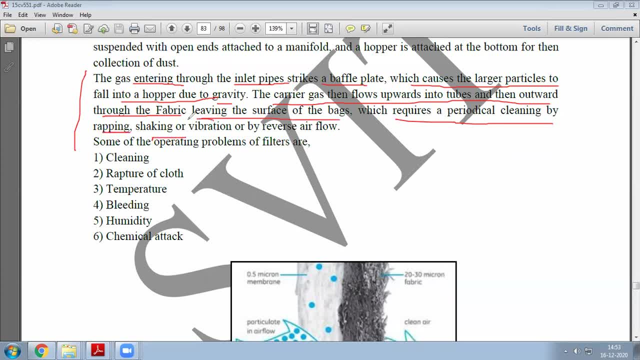 periodical cleaning by wrapping, shaking or vibrating. so it will be vibrating, right, so all dust will come and uh at the bottom and uh, all clean air will go up. so sometimes they will reverse the flow or they will vibrate more or they will shake more to clean this. okay, so that's the function. i will move. 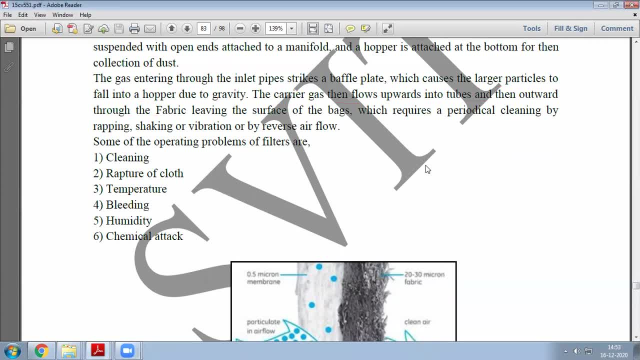 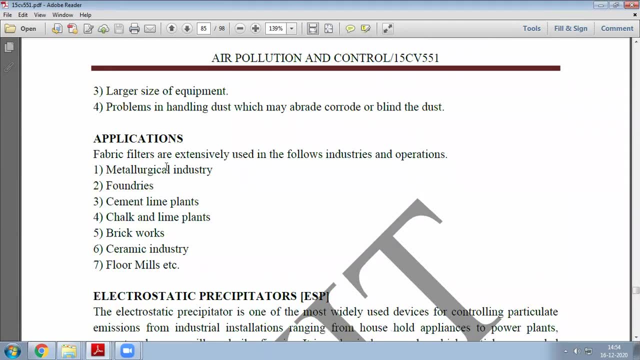 on quickly. what things are there? so, yeah, one thing is those two things i have done. this advantage is not that you right, try to read. application means where and all. it is applicable: industries in metallurgical industry, foundries, cement, Charles line plants, they're all. they'll use this thing. okay, next, one more you have 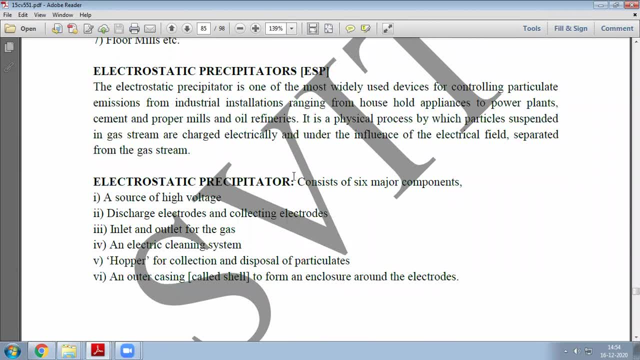 electrostatic precipitator is very important. wait, i will try to call yes. so electrostatic precipitator. so you know the terms. electrostatic precipitator means something it is arresting due to electricity. that name request itself will tell some: electric energy, electric potential generate. 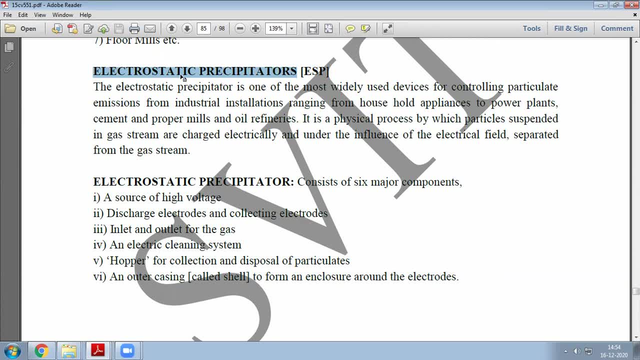 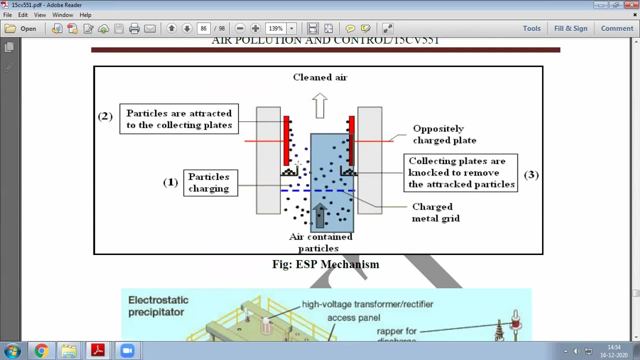 it. that will help us, to you know, hand or arrest any of the particulate or any of the pollutant discharging in any industry. okay, so how it looks first i will tell general way. see, here they are creating some potential difference here, right? so what two electrodes they have. 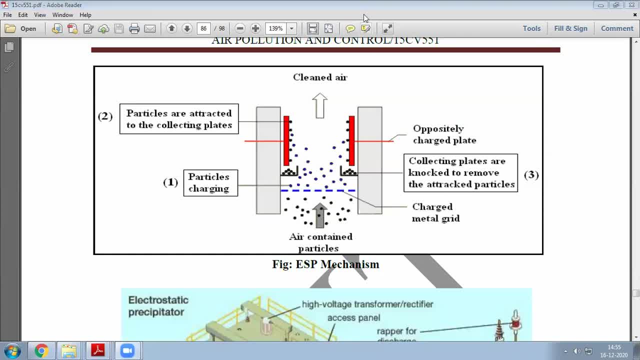 placed. when two electrodes are placed, some potential difference you will see right here the two electrodes you see one is here, one more here, so it's arresting some, it's creating an electrical potential. because of that, what happening? particles are charging and some, some particles are collected here in the electrode. 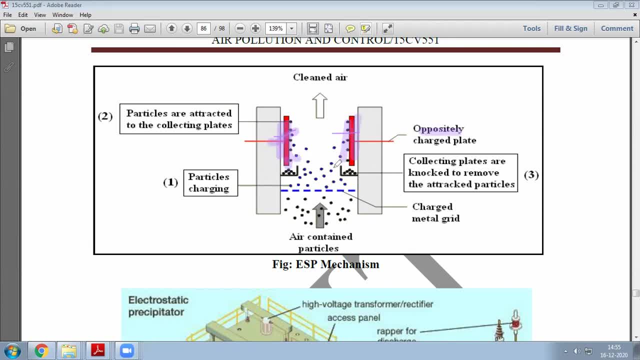 and that is nothing but oppositely charged by charge plates. because of that charges attraction, it will collect here all particles, they will be collected here and and clean air will pass through this. okay, so the potential difference makes you makes makes all all the particulates to collect and be there in the electrodes only. okay, that. 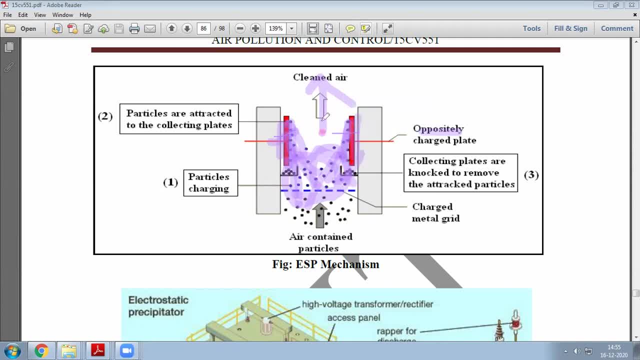 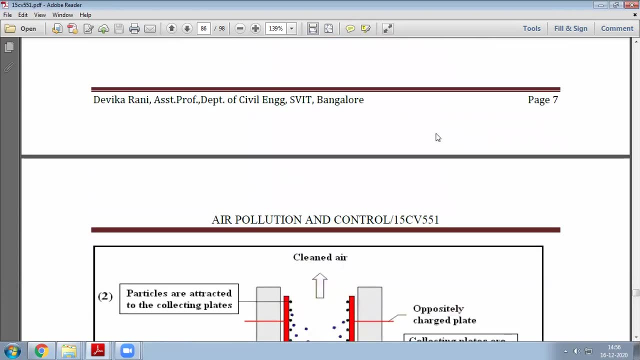 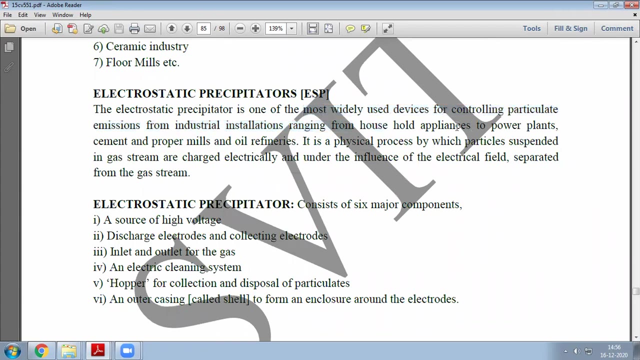 is the principle and clean air. obviously it will move in the upward. here, clean air will move upward, so this is the function. so we will go through this pdf now what this tells. electro cycle precipitator is one of the most widely used in where and where in cement paper. 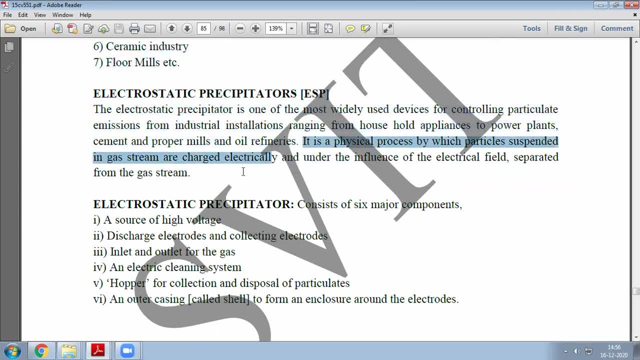 mill oil refining. it is a physical process by which this is a process up to here, physical process by which particulates suspended gas stream are charged electrically and, under influence of electric field, separated from the gas stream. so i already explained in general way you go through all this thing. 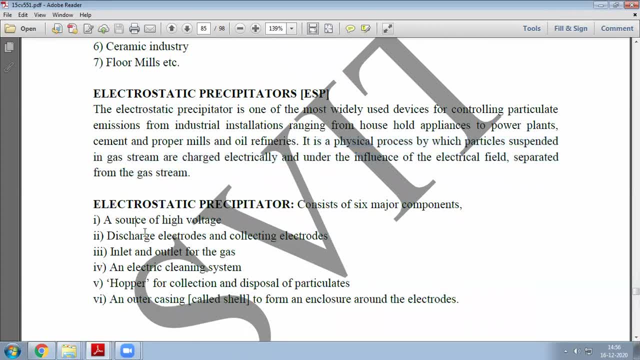 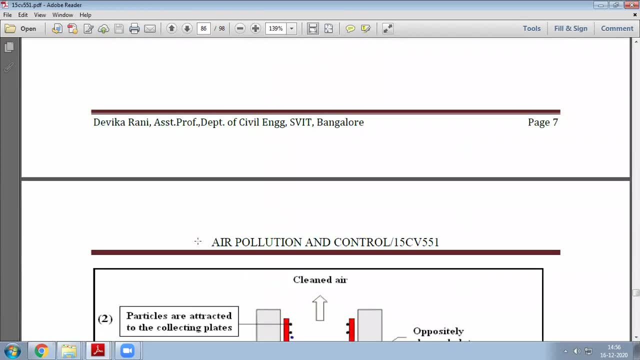 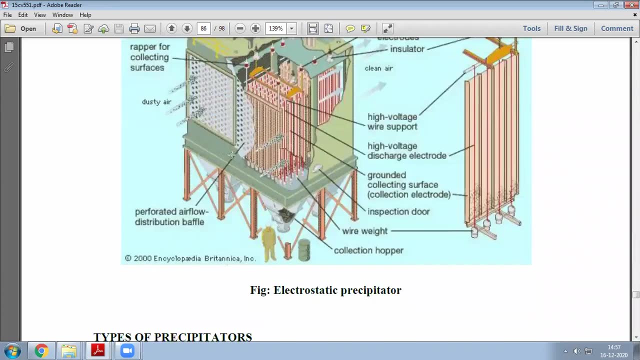 this is nothing but what and all it contains the figure it has: i: electric voltage, discharge electrode, inlet, outlet, gas, electric cleaning system. you go through all this thing concept. i think i already told you this is how it looks. don't write this figure in the exam, just write this one. 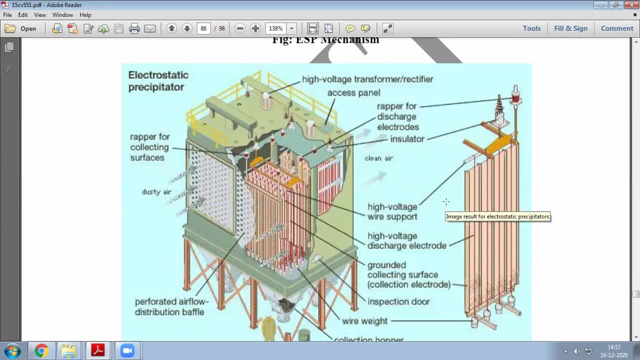 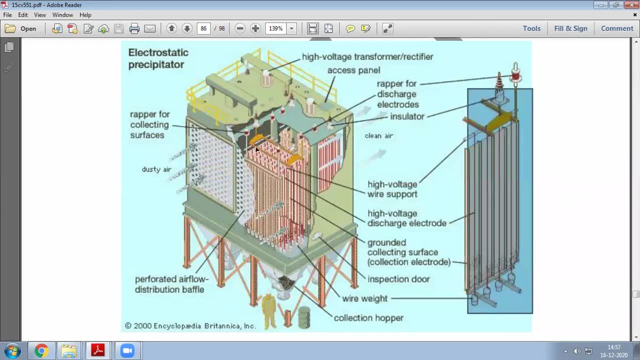 so see here, here is the free electric field which is charged electrically and under influence, how it will be seen in the industries. this is all the collecting electrode. uh, they will install like this. if you see the cross section, it has nothing but so much of electrodes only right. so here the stair is going in this side. 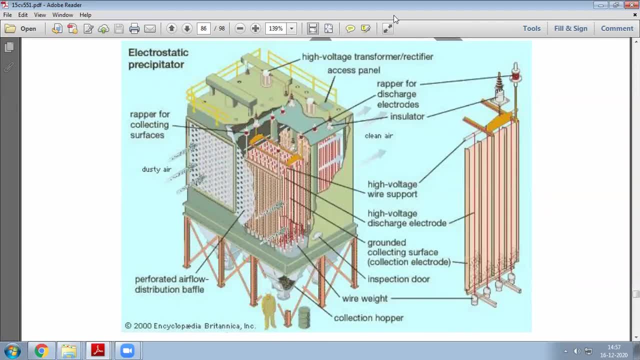 yes, so the stair is going like this. but when you cut this into pieces, you're seeing what this electrodes- a lot of electrodes. so they are arresting each of the particle. okay, it's moving like this and, uh, it's moving like this and clean air is coming like this. so 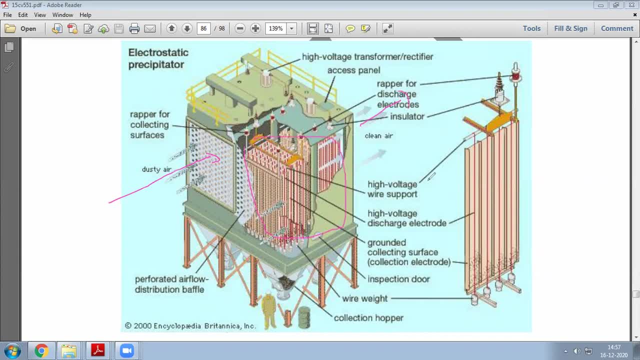 all electrodes, so many electrodes they have installed. so this is how it functions. okay, the concept is what? uh, the electrodes made up of oppositely charged, so obviously they will attract each of the dust, air, particle, particulates, and clean air will be passed like that. okay, 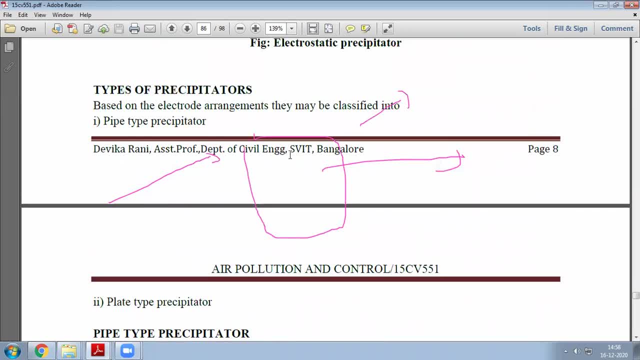 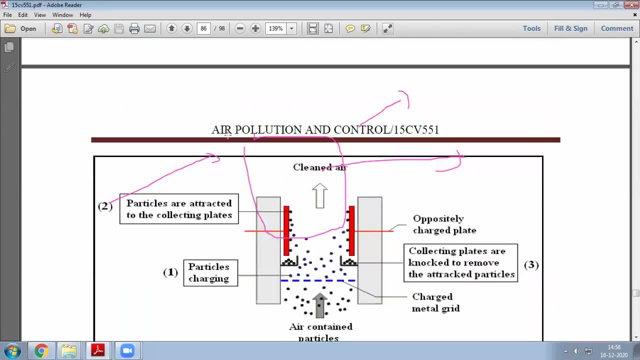 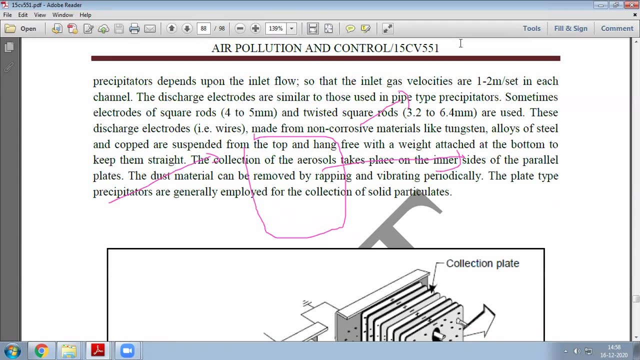 so one more you have. uh, actually there are two types of this electrode precipitator- those things you don't need, uh, you just read this one. only this is that off. they are classifying this. actually. they don't ask: this pipe type esp you have, and uh, 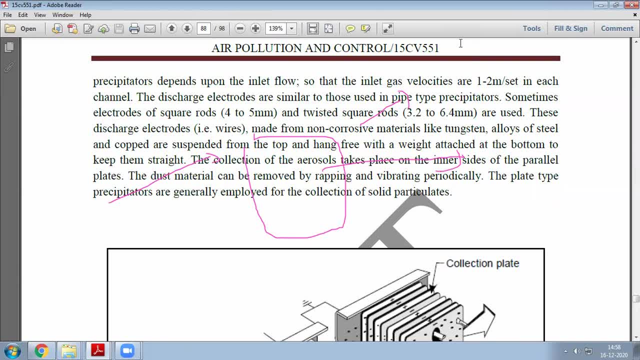 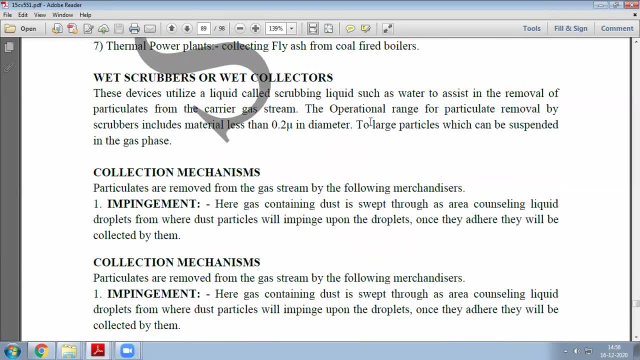 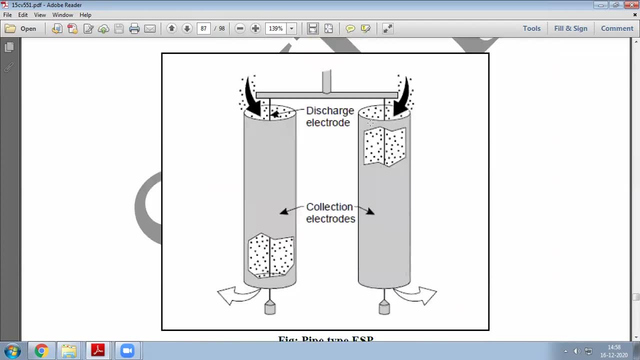 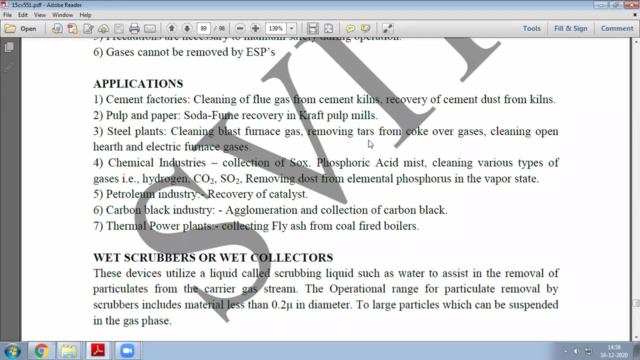 okay, wait, yeah, so you have pipe type and uh, one more. you have uh, closed, one more. you have plate type, plate tape and pipe type. two types are there. don't require, you don't require this directly. you study the next thing important, but you study all this advantage, disadvantage. 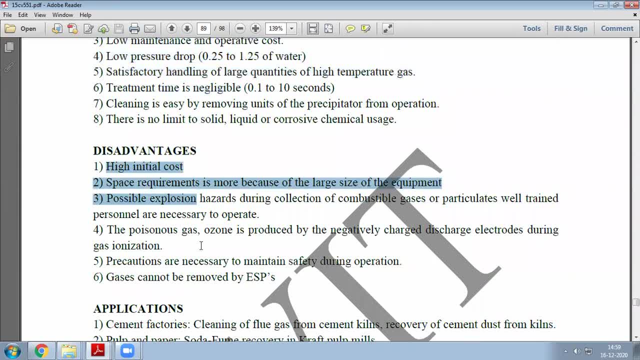 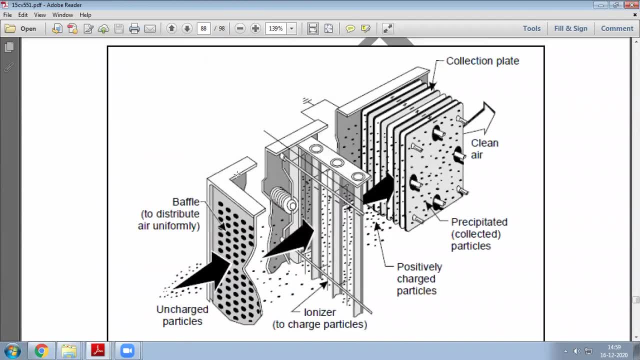 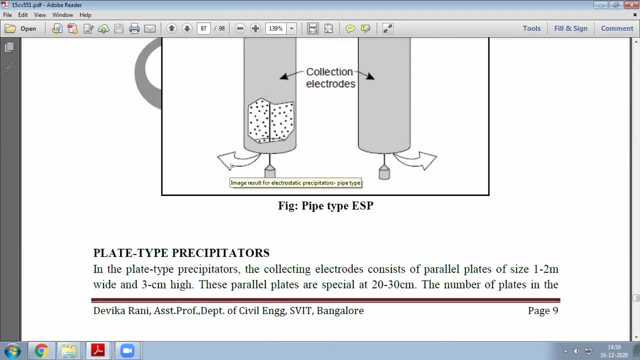 these are all important. what are all it removes and what are the problem we will face like initial cause: space requirement, okay, those thing you read. uh, okay, they just classify this: either pipe type or plate type. it means the electrode, if it is in pipe type or it might be in a plate type. 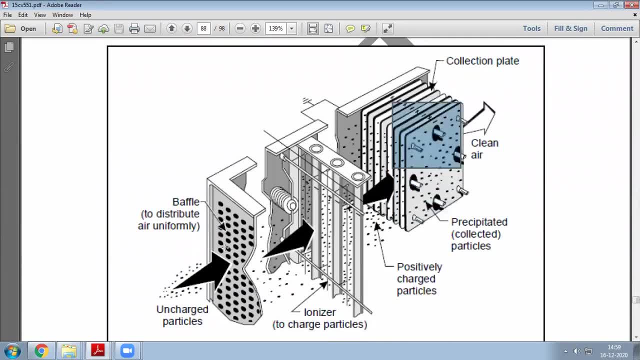 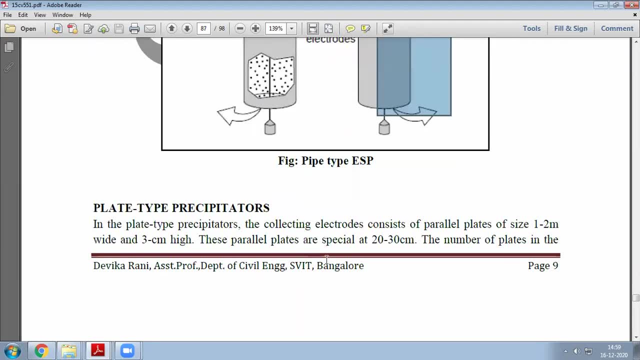 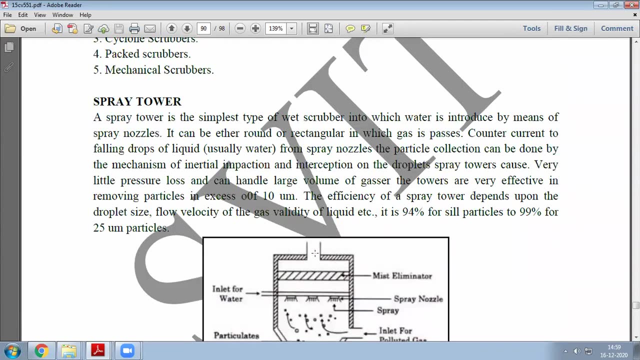 plate type. it will look like this: see, this is all plate type and this is all pipe type electrodes. okay, so it's nothing but the configuration of electrodes. so you go through this. i will show you when i give you further. So you go through this. I will quickly go to next concepts. 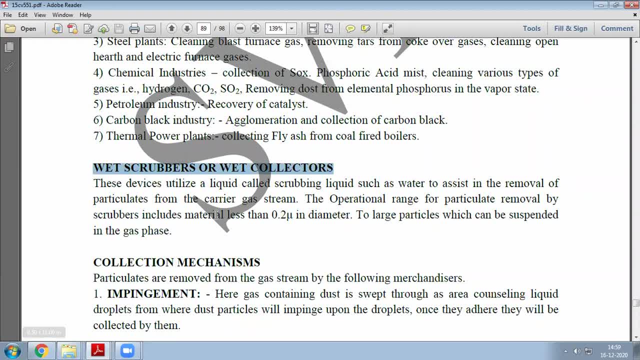 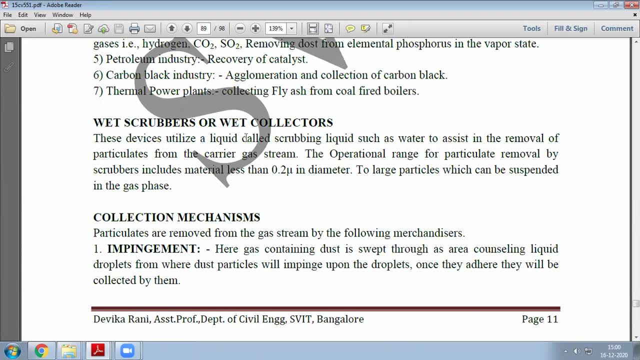 So this wet scrubber is also important, or wet collectors. So one more concept: is there wet scrubber, or wet collector we call? What is this then? this device utilized a liquid called scrubbing liquid, such as water, to assist the removal of particulates from carrier gas stream. means it will utilize 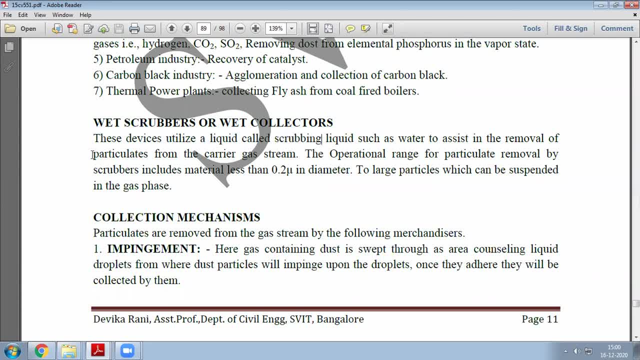 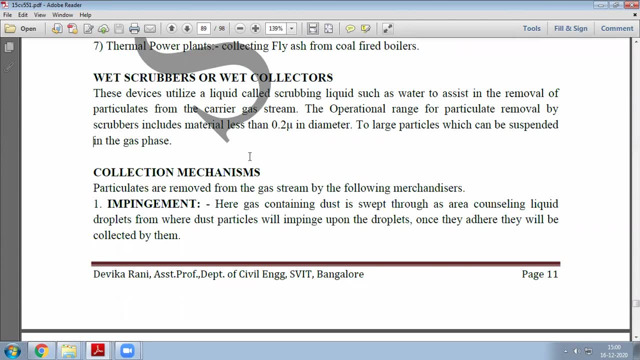 some liquid like water, and this will help to remove any particulate gas or carrier gas which was there. So how much it can remove means 0.2 micrometer in diameter to up to a larger particle suspended in the gas. up to that it can remove. 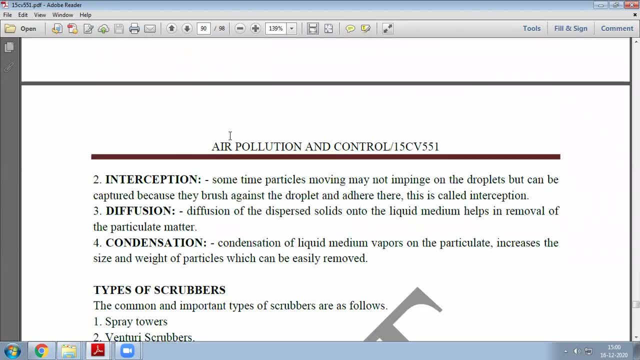 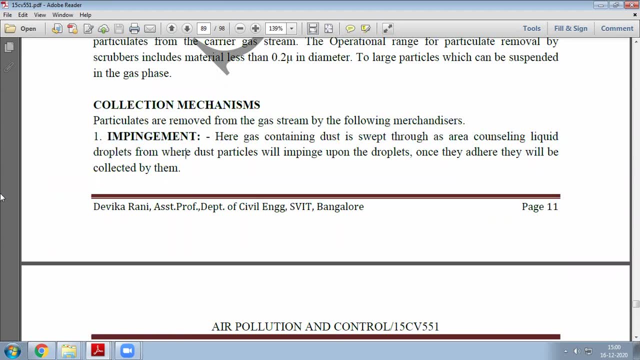 So how it will do that mechanism. So this is what they have given here, around 4 they have given impingement was first thing. What is impingement Here? gas containing dust is swept through an area concealing liquid droplets, from where? 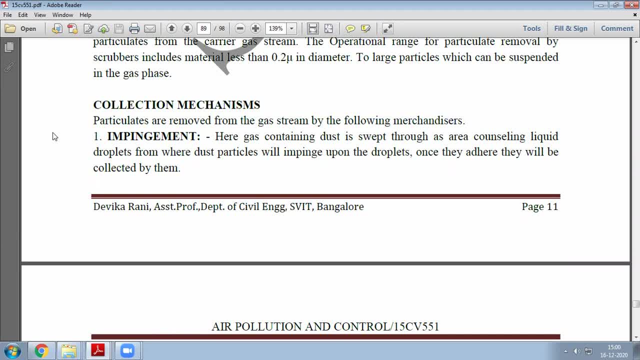 dust particles will impinge upon droplets. once they adhere, they will be collected there, Means, since it is a liquid right. so all gases try to, you know, impinge upon droplets or on the liquid which was there, like water. So they will try to impinge on the liquid available. 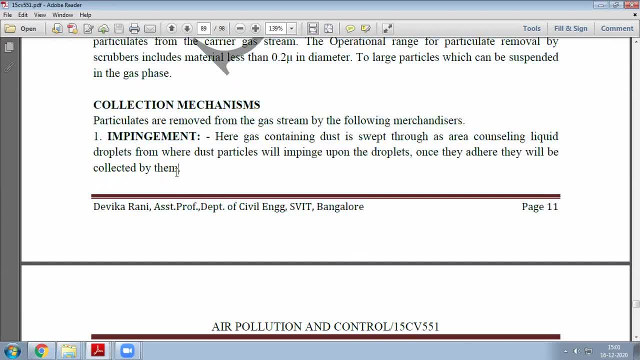 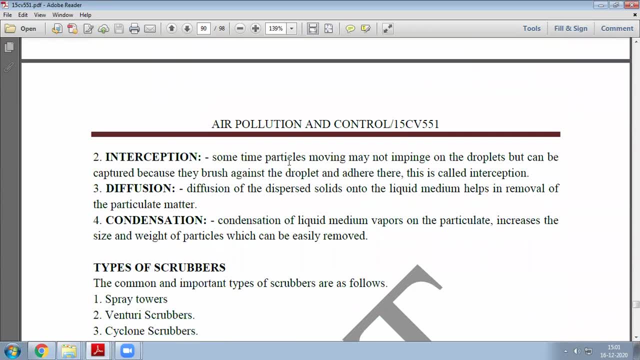 Once they adhere, they will be. they remain there only and we can collect it back later. Next you have one more type like interception type. This is particulates moving may not impinge on droplets. Sometime if it doesn't adhere or impinge on droplets, but it can be captured because of. 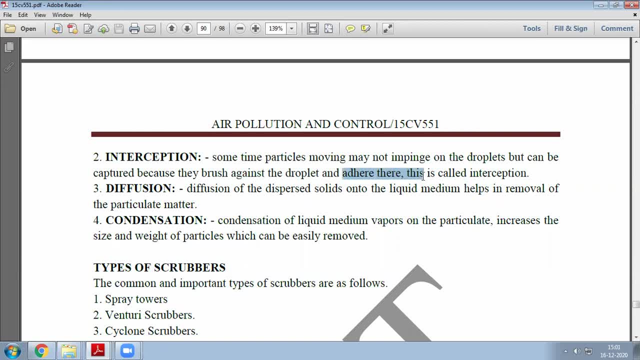 the brush against the droplets and adhere there. This is called interception, Interception. Interception means if it is not impinge there then but also it will try to adhere. by the process called brush or any of the you know, going against to the droplets, it will adhere. 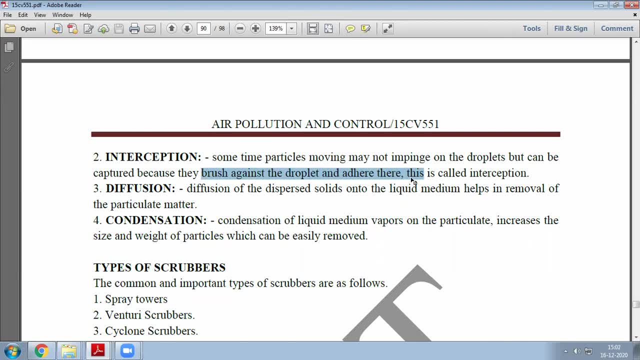 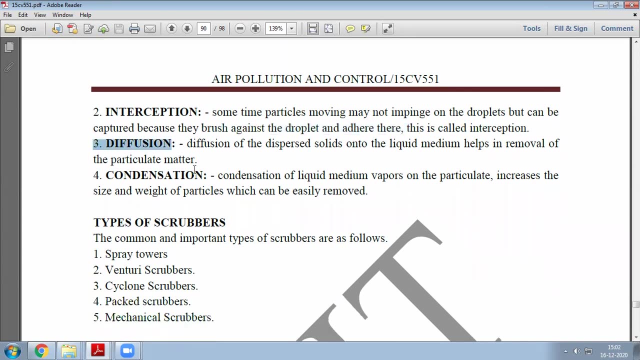 there even the liquid, not in an impingent, not so adhesive it, because the particulates anyway going to that liquid right. So that is interception we are calling, because of that also we can reduce. Next you have a diffusion. Diffusion means, you know, disperse solids into liquid medium. instead of two phases happens. 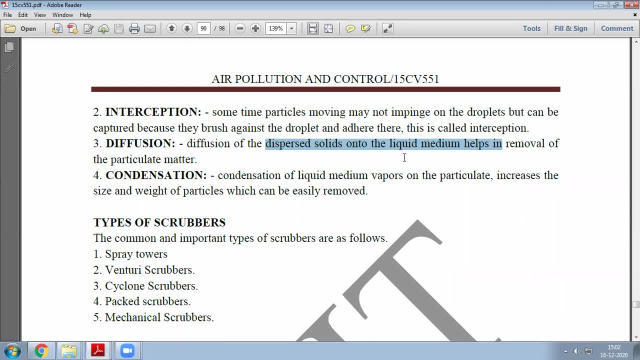 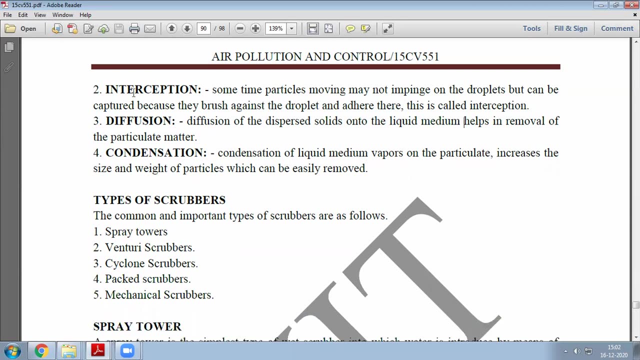 here solids and liquid. the disperse phase is solids and disperse medium is liquid, just like your Colgate you are seeing now. so it's a diffusion. so all particulates will be diffused. that is also one method. Next you have condensation. condensation of liquid medium vapors on the particulate increase. 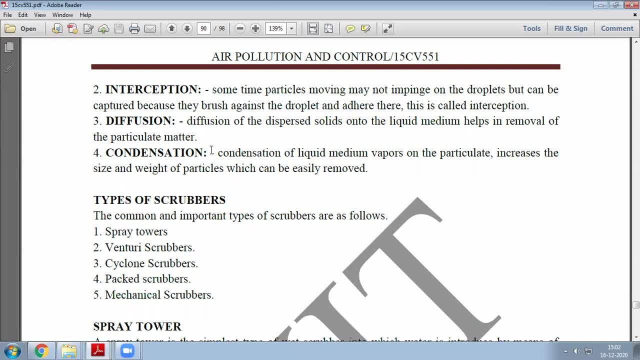 the size and weight of particulate which can be easily removed means condensation, means what we want to condense: the liquid, okay, vapor, or then gas. so obviously size, weight of will increase and after that we can collect it and remove, okay. So all the theory they have given here, mechanism means 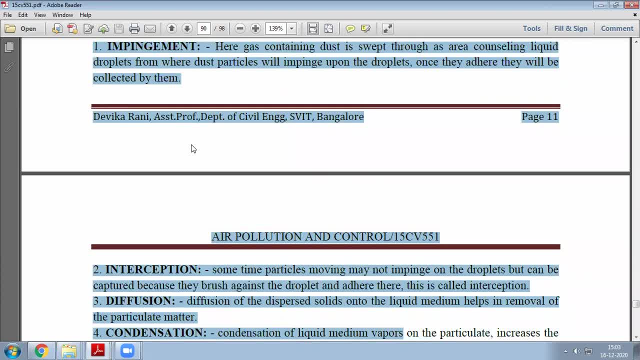 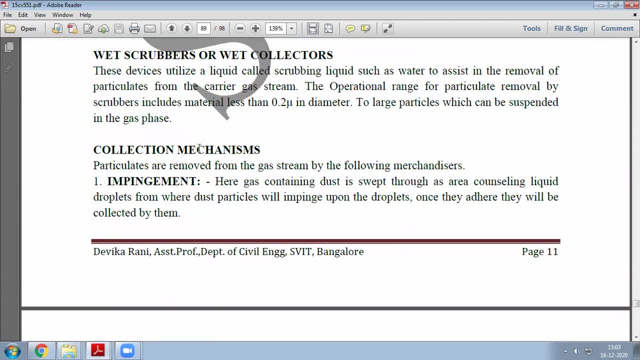 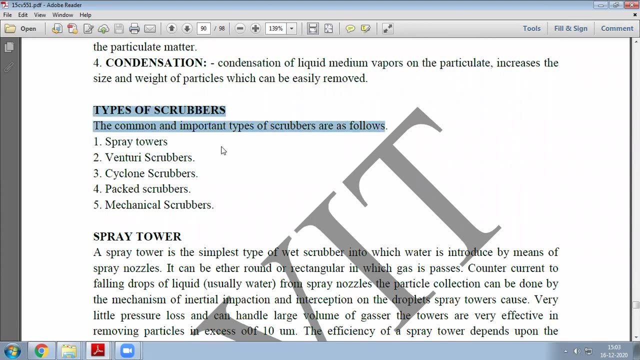 Any four mechanism, it will fall. any of the four, it will fall. and that is how, because of the impinging, this wet scrubber, removed by those that liquid that they provided. okay, So now, what are all the types available in the market? you have around four to five types. 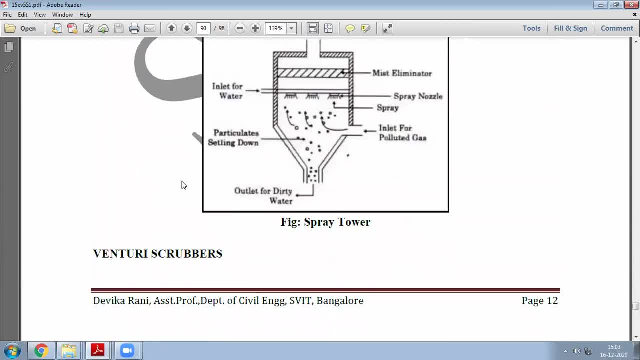 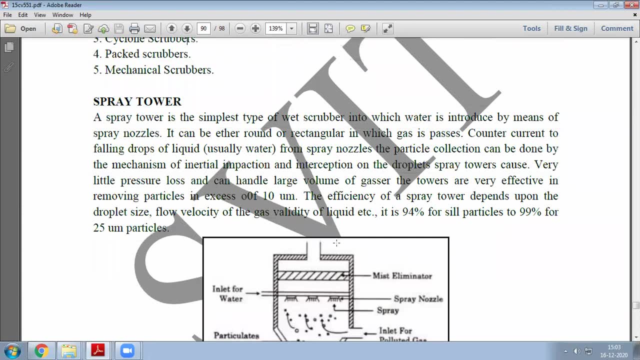 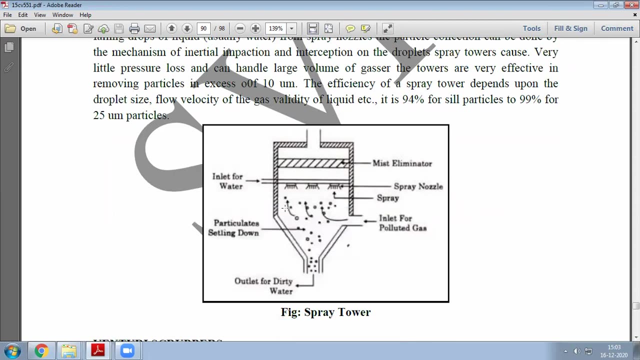 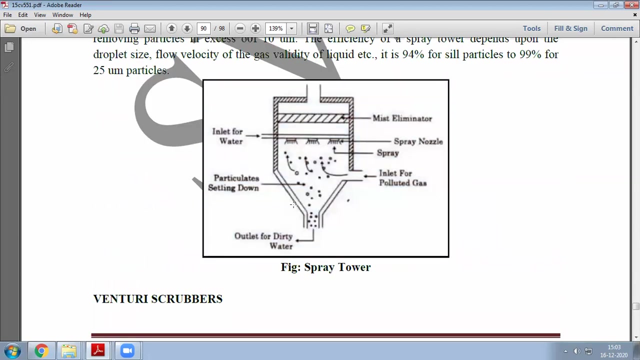 straight over ventures, scrubber, cyclone scrubber, like that. So yeah, So all works in this Same fashion, only same theory. okay, So just see how the liquid is passed here. so that, what making difference here with respect to spray tower? if you see the figure itself, the particulates are settling here in later. 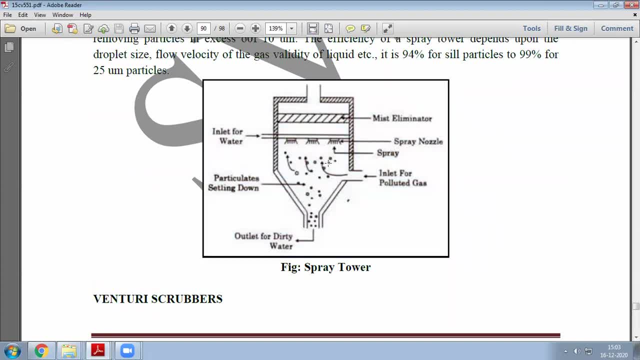 water will be sprayed like this. if the spray nozzles is there, because of this liquid, the gases are coming now it will be arrested. the particulate will be arrested here and pure gases will pass. So that is the mechanism. so spray towers is the simplest type of best rubber in which 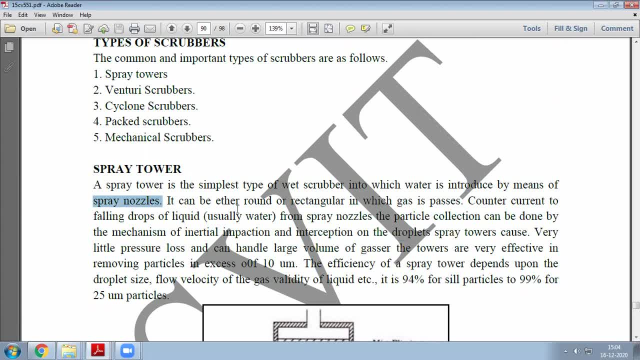 water is introduced by means of spray nozzles. it can be either round or rectangle. which gas passes, counter current, falling drop, liquid sprays nozzles, the particular can be done by mechanism. so same mechanism, same, like interception we have gone through now. so that mechanism. 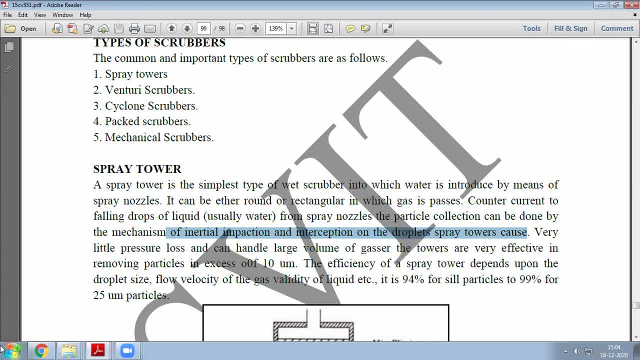 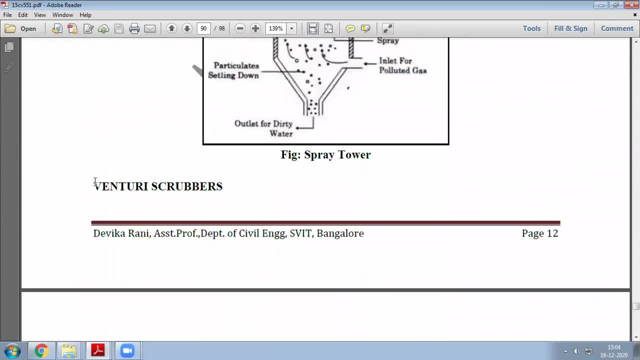 only it will be removed here. the methodology is what they are Supplying the liquid in spray. okay, so that is the term they are given as a spray tower. next one more. we have venturi scrubber. what is this? so, venturi meter, you have studied? 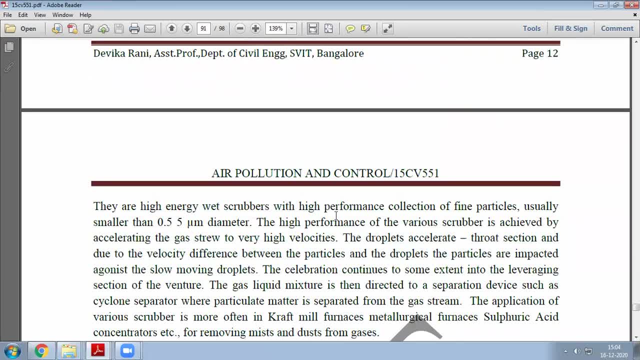 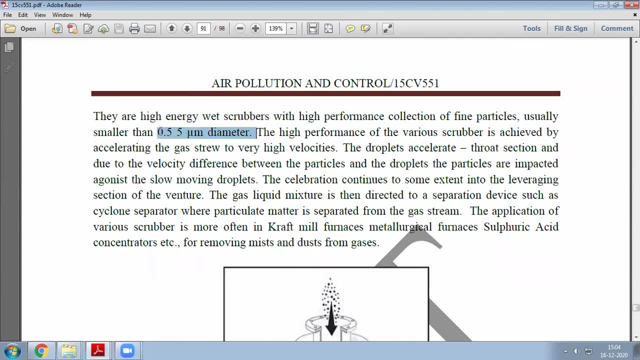 in the fluid mechanics. it's similar to the shape. that is why they are given, so we will go through this then. they are high energy wet scrubber with high performance collection. fine particle up to 0.5 to 5 micro meter diameter. So here how the droplets are arrested. 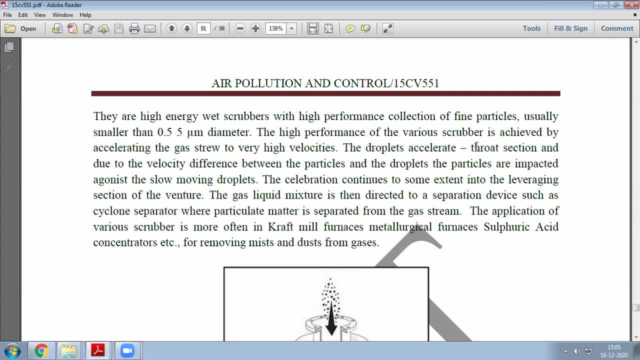 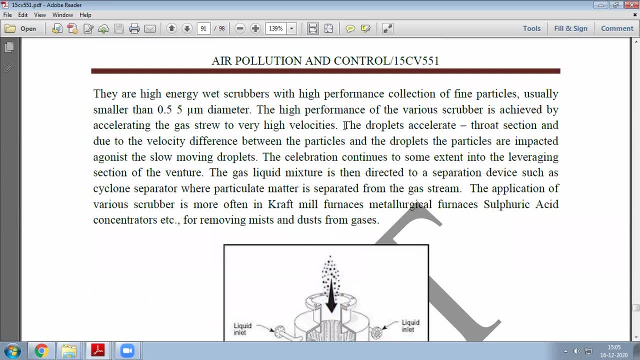 The droplets accelerate throat section. throat section means this section. you're seeing this is called throat section. the droplets accelerate means all the droplets will come here in the throat section and due to the velocity difference between particles and the droplets of the particles are impacted against the slow moving particles. so there is a liquid also there. 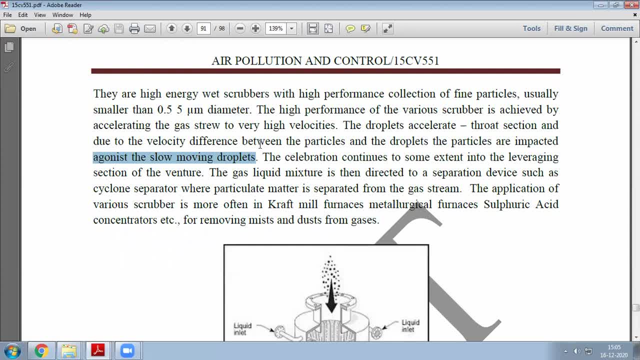 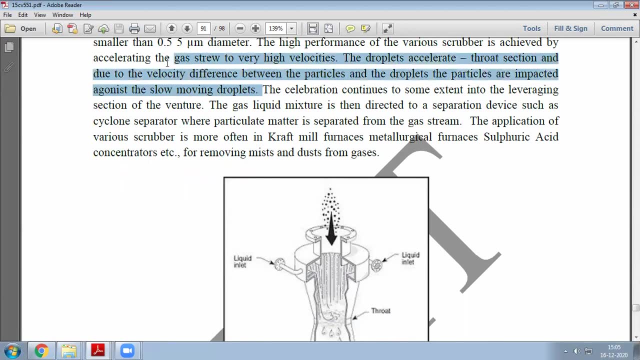 and gases also there. So there is a difference in what Particles, velocity which they're coming. okay, so there is a difference. because of this, The all the particular particles are settling. okay, so that is the concept. up to here. you remember and write, and write the figure, this and all you don't require. so I will move on. 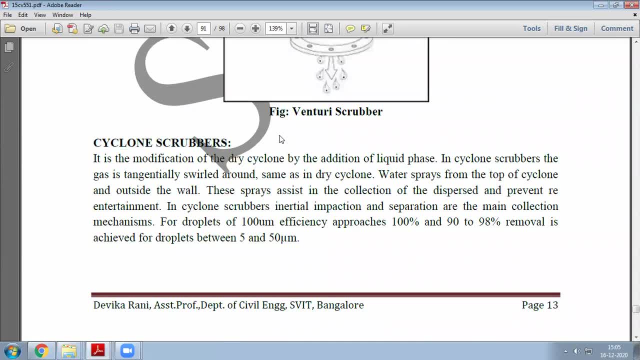 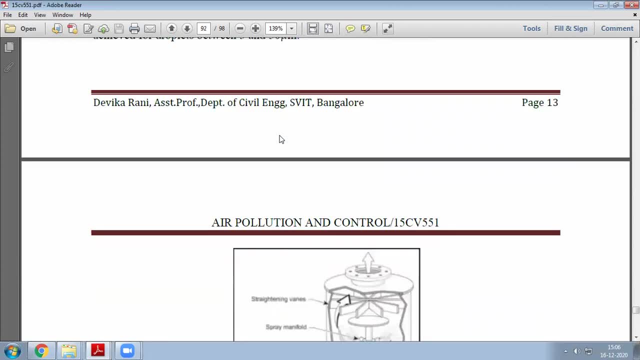 to one more cyclone scrubber. it's also same phase. it works in the same principle. okay, wet scrubber means some liquid will be there. it will be arresting, Okay. So how it will looks is like this: see here: water in, water out, spray how they're spraying. 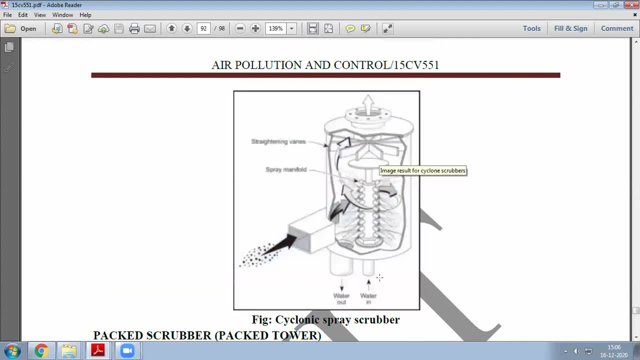 the water. there is a straightening. wins is there, water is coming here, water is going here, but here all dust is coming. water they're supplying from the bottom and dust is apparently there. it is going. so a lot of mixing is going here. here. clean, clean air is passing like. 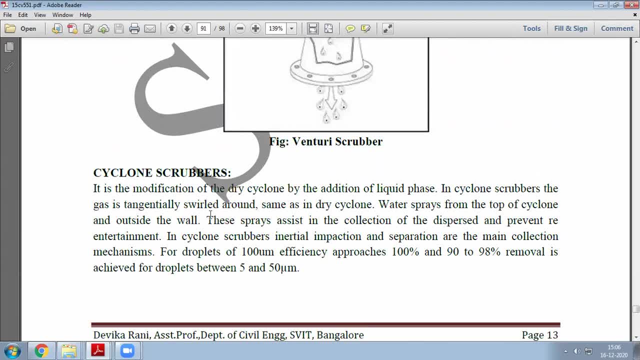 this. Okay Now. cyclone scrubber is a modification of dry cyclone by addition of liquid phase. cyclone scrubber where the gas is tangentially spilled around the same dry cyclone: water sprays from the top of the cyclone and outside of the wall. this spray assist. this is important mechanism. 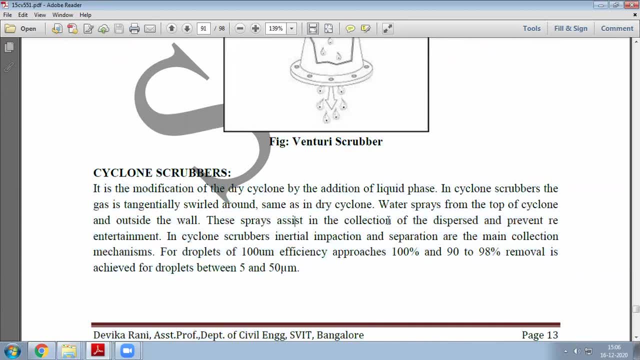 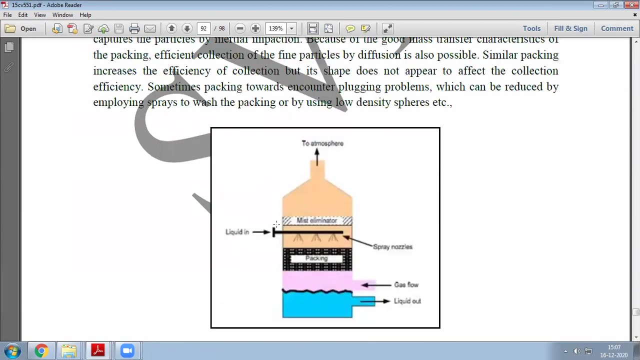 this spray assist the collection of the dispersed and prevent re-enternment, so it will arrest their telling. Okay, So that's over anyone they might ask. or you just have to study the diagrams. after that you can write on your own, because once you remember the diagram, you can just try to elaborate. 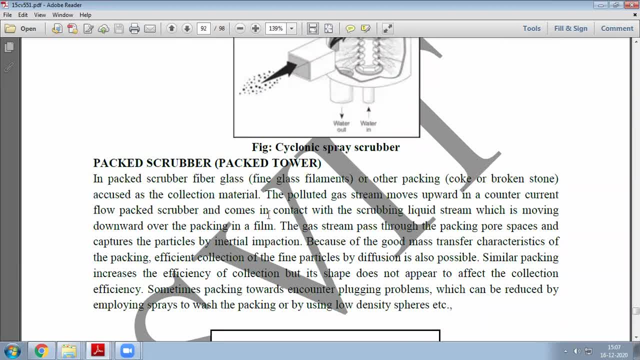 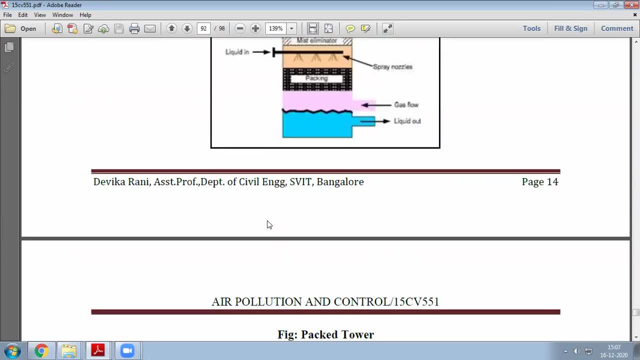 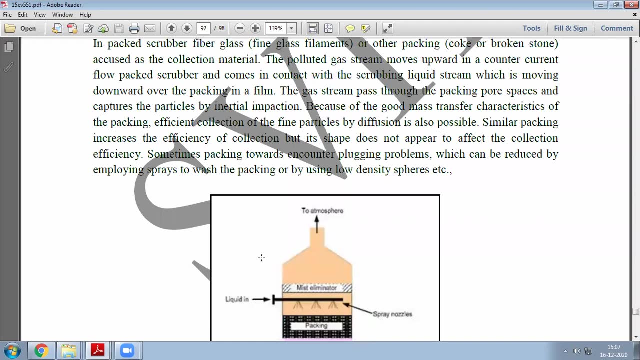 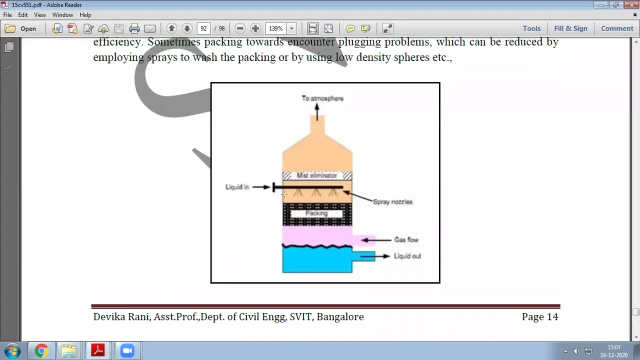 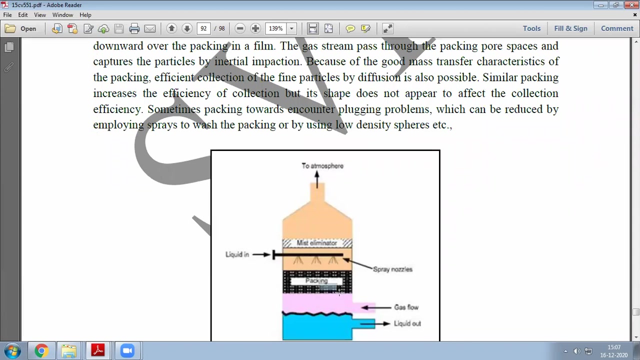 that, okay, Okay, Okay, Okay, Okay. So one more: you have packet scrubber and what else is there? yeah, this is the last typing your fourth model. this is the last topic packet scrubber you have. you will see that what it is packing is there. yeah, so liquid is passing like this. some packing material is there here. 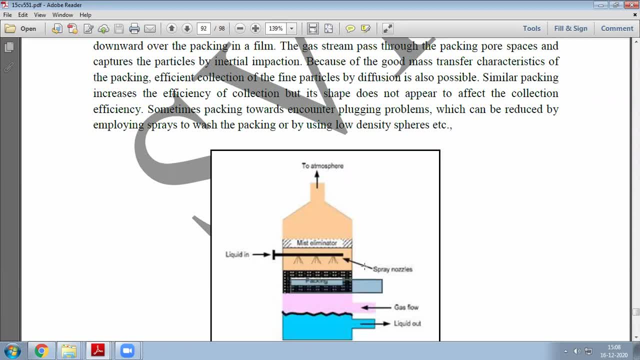 you're seeing the figure right. just seeing the figure, you can observe what happening here because, since you know, the concept is nothing, the liquid will be there. that is going with all the four mechanism theory. we have seen no interception. is there impinging activity is there? so any of the thing? it will fall and it will remove. so that is the theory you. 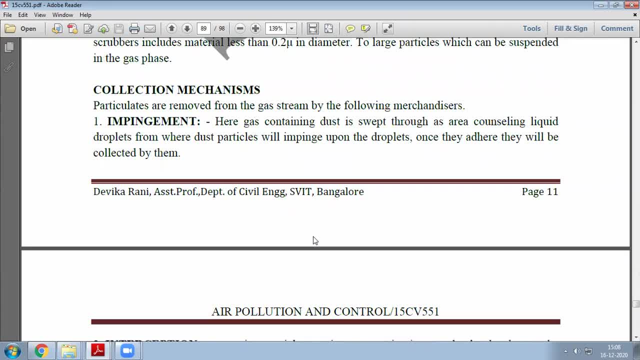 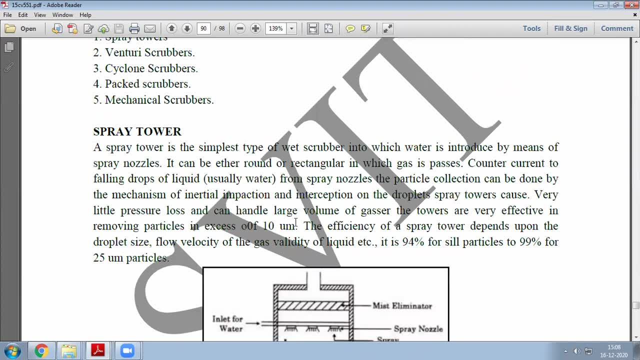 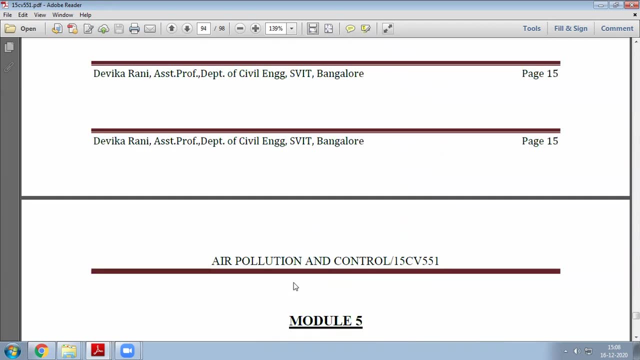 already seen here. right theory have gone through. in the first only see impingement, interception, diffuse and condensation. Any of the four mechanisms, Any of the four methodology will be there in all this scrubber. okay, all the works in the same principle, but just how they will made it that's making the difference. so last, 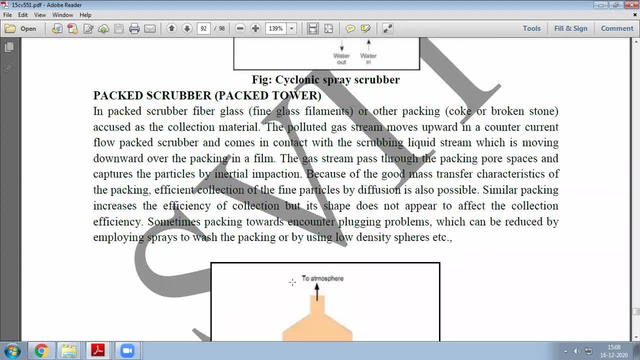 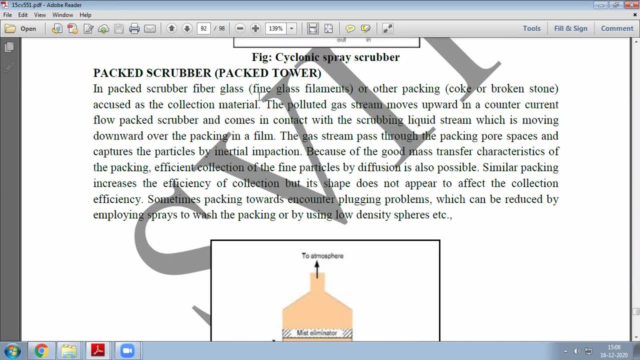 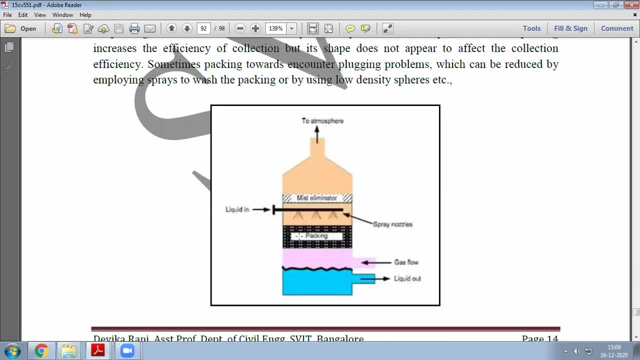 one thing is remaining. this is packet scrubber or packet tower, so I will try to do that now. okay, the packet scrubber, or fiber gloss or fine gloss, filament or other packing or means they are creating some material here, packing, you're seeing no, so it has made up of some. 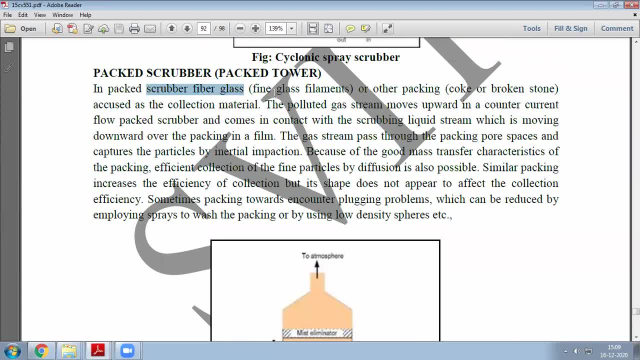 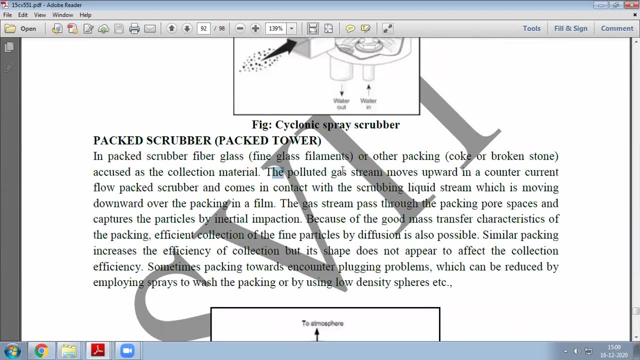 materials. I'm reading now see this. it made up of what? some fiber glass or fine glass filament or any coke or broken stone. okay, don't material, they'll fill it here. okay, so the polluted gas tree moves upward in the counter current flow packet, scrubber and come. 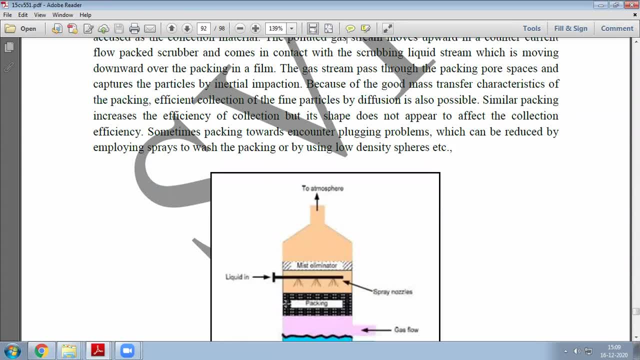 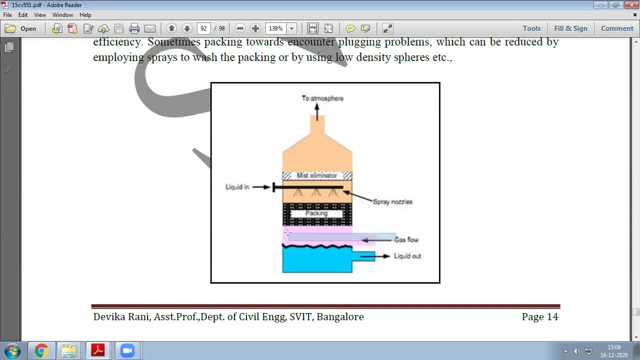 in contact with a scrubbing liquid. yeah, see here gas is coming. like this gas flow is happening like this and it will come in contact with sprays already supplied in the top liquid in liquid they are supplying like this: wait one minute. yeah, see here our gas is entering. 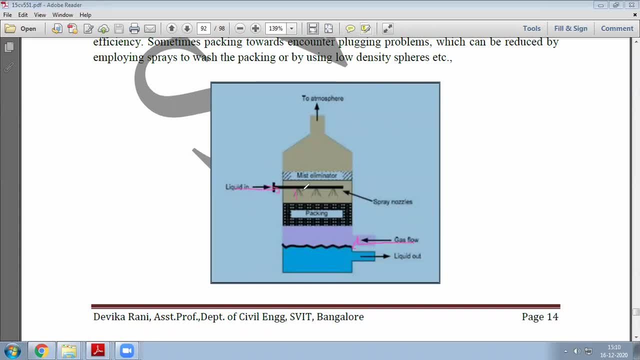 like this and liquid are passing like this. Okay, Okay, Okay, Okay. So there is a packing material made up of some glass or any filament. So, because of this adenosine thing, all particle will be arrested here. okay so, and all the 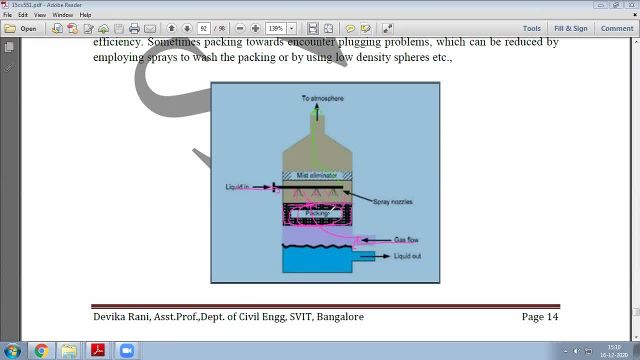 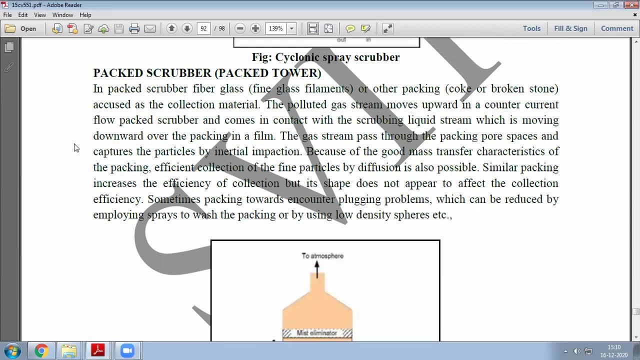 clean gas will be gone like this. okay, so that is all what they are explaining in the PDF. see here, yeah, here the gas stream. from here it start. The gas stream pass through the packing pore space and captures particle by inertial impaction because of good mass transfer characteristics of the packing, efficient collection of the 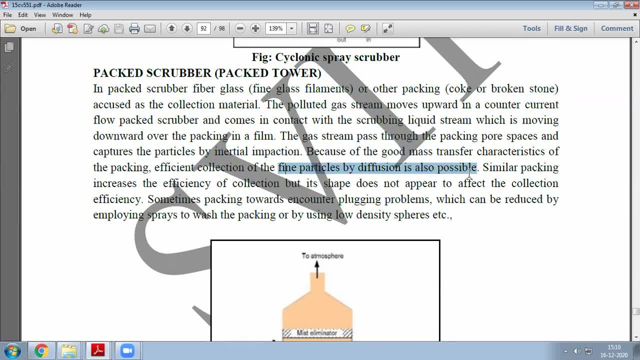 fine particle by diffusion also possible. the fourth method, your third methodology, has studied no diffusion and already you know impaction, the second, or interception, that also. so any of the three, four thing, two things are going here because of this two mechanism theory or any mechanism. these gas are removed, water on the mechanism by diffusion and inertial. 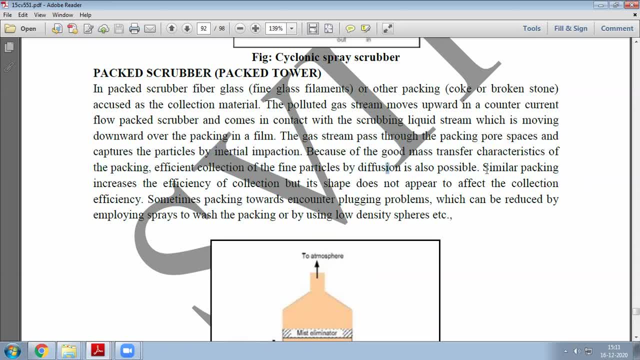 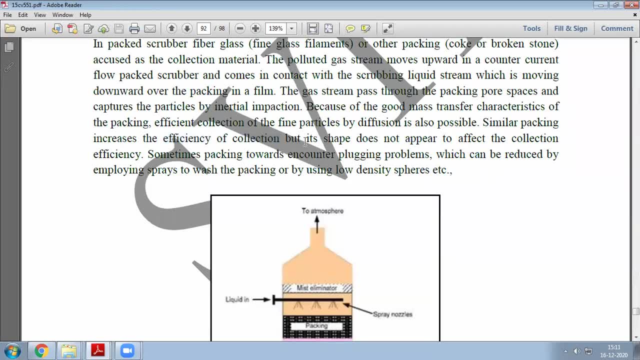 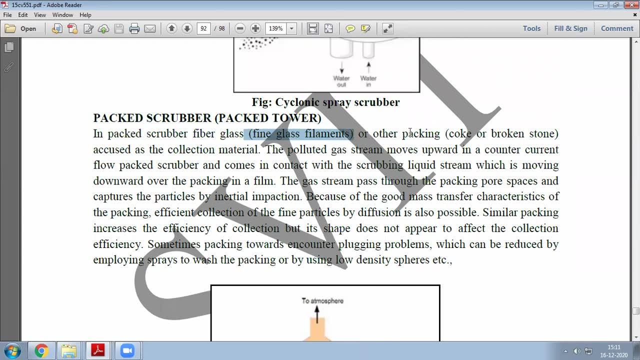 impaction. So because of this the gas particulate are removed. similar packing increases the efficiency of the collection. So additionally they are speaking- means more packing of the materials, of this fine glass filament or any other coke or broken stones. We can increase. what efficiency in the collection. 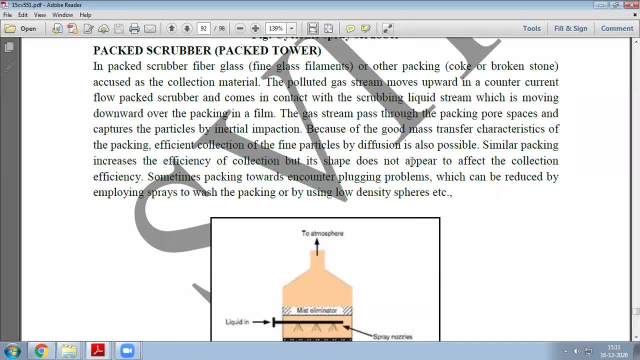 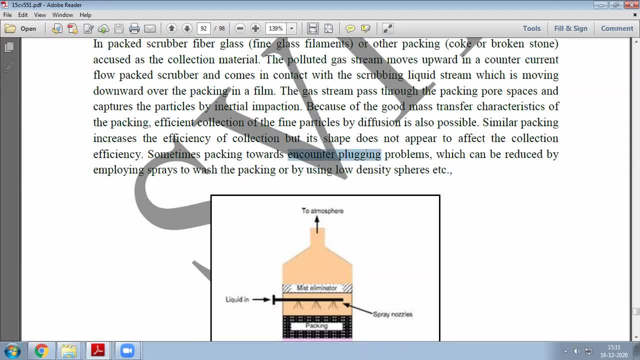 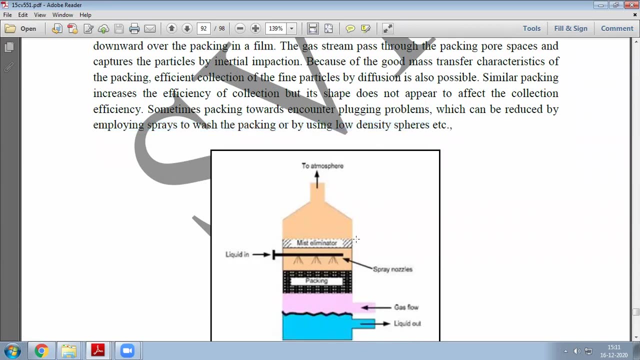 It might be anything, Okay. So sometime packing tours encounter plugging problems, which can be reduced by employing sprays to wash the packing or by using low density sphere in some plugging problem might be there. So that is why they are supplying constant, you know, liquid or spray. 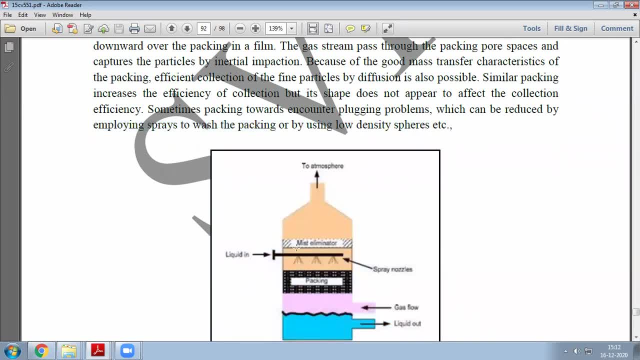 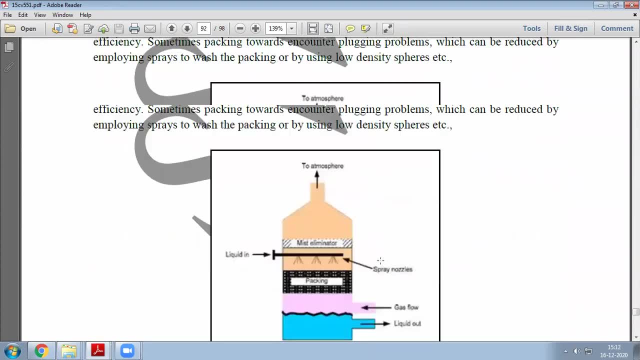 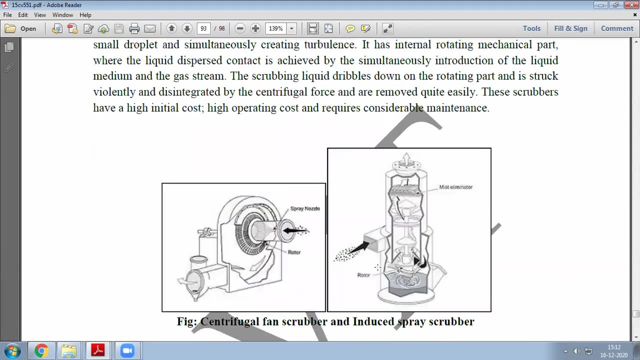 here they're supplying the spray, so that will eliminate any of the problem that might arise. okay, so, yeah, so that's about packet scrubber. uh, what else you have? mechanical scrubber. one more is there. last one, i think mechanical scrubber also there. so we'll try to see that here. what? 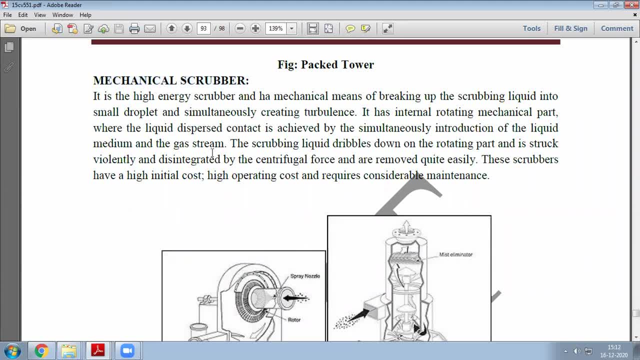 is mechanic. all are works in the same principle, around five to six years study. no, it's the same theory. some liquid will be there and some some. you know, at the end you have came out some packing material, all they are designing. so they are both combination, all particulate or any pollutant. 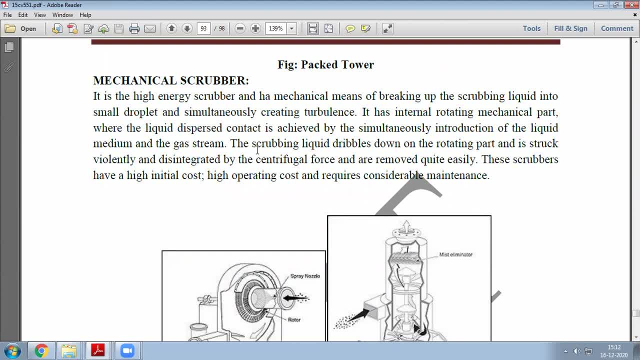 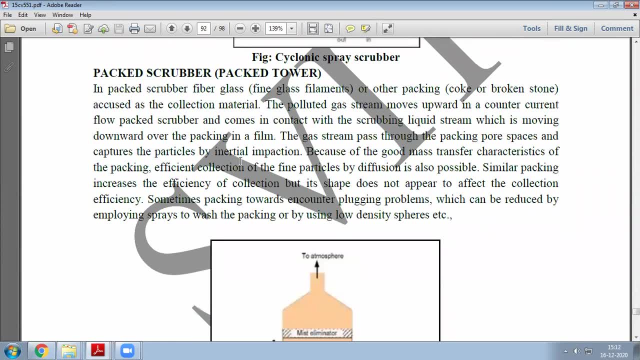 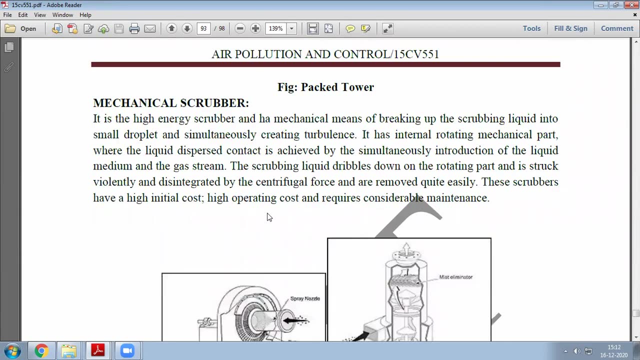 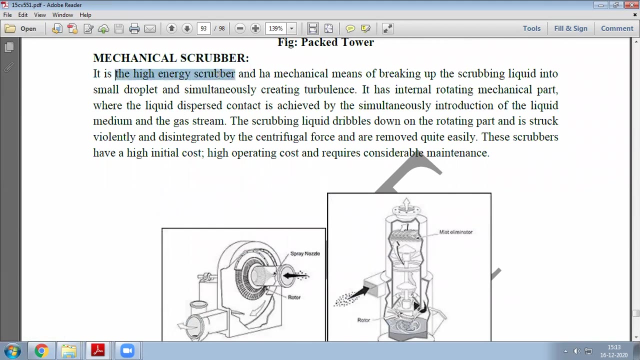 which is in the air, it is disappearing, it is arrested by that. okay, so we will see. last one is scrubber, this, this. only what is the mechanism they are talking about? what is the mechanism of this scrubber? scrubber, okay, okay, so it is a high energy scrubber. mechanical means breaking off, scrubbing. 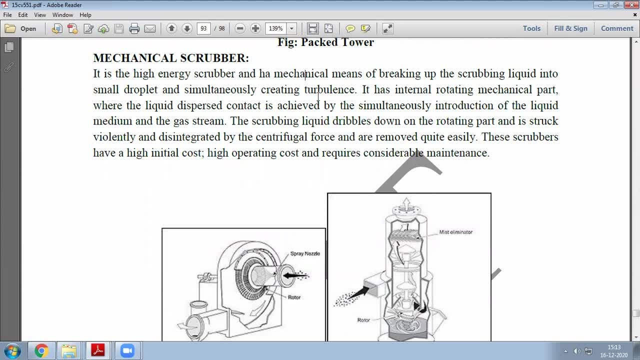 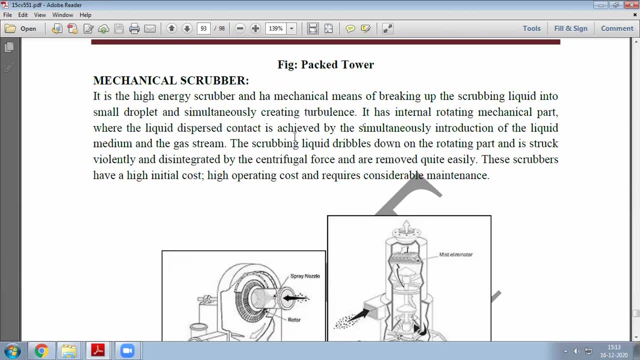 liquid into small droplets and simultaneously creating turbulence. so one more high energy scrubber. you have wet scrubber we call uh. what it doing here? it breaking up the liquid into small droplets. whichever liquid we have using here, no, it will break that into small droplets and and with doing that it also create. 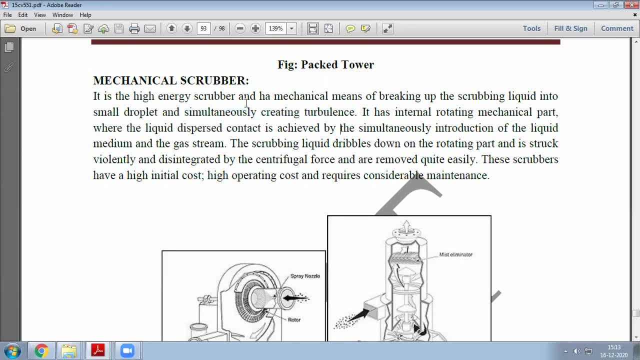 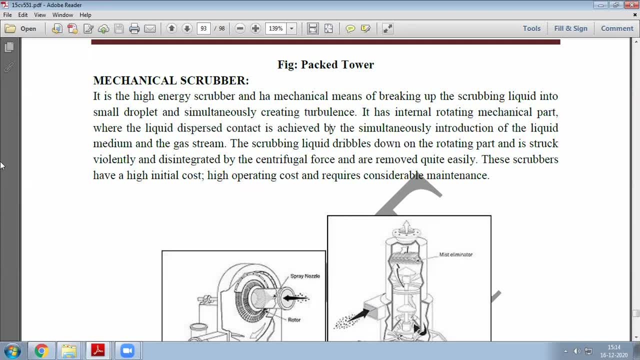 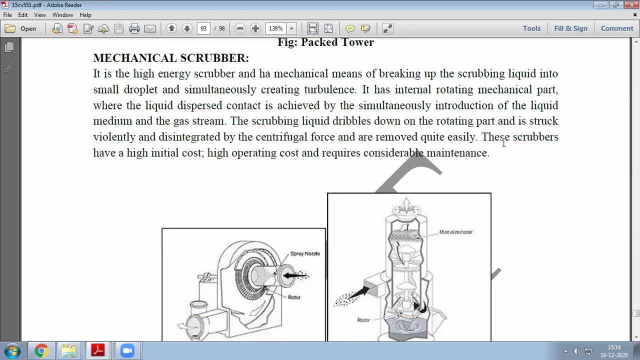 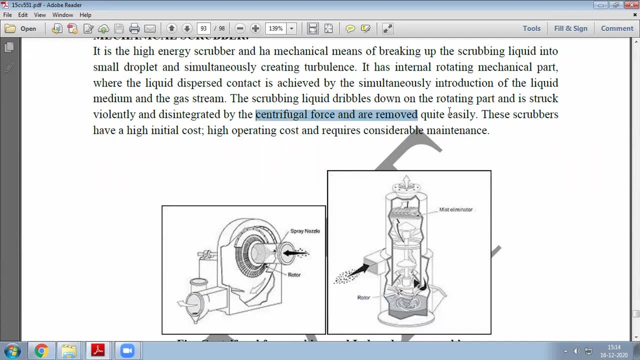 liquid drip dribbles down on the rotating part of and uh is stuck violently and disintegrated by centrifugal force. so centrifugal force- if you're interested in watching this video, we will arresting the movement also once the centrifugal force we have introduced. no how this force is moving like that, only all the deposition of the particulate matter happens. 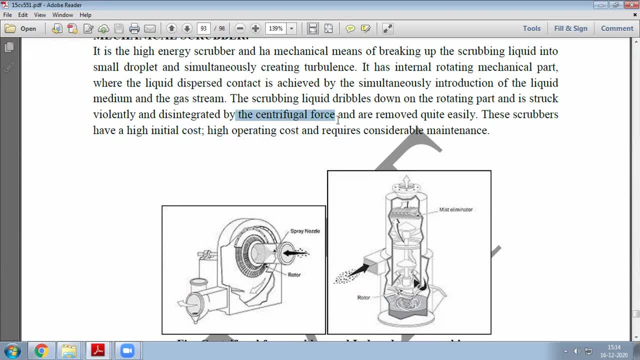 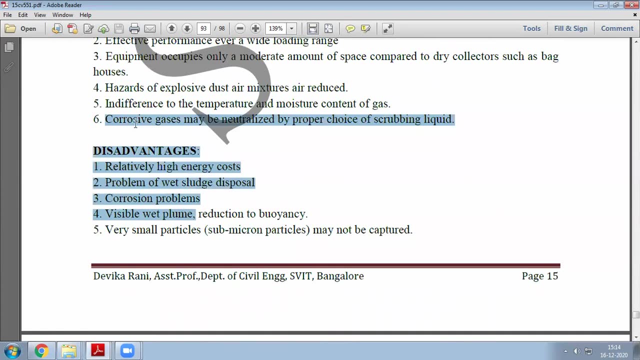 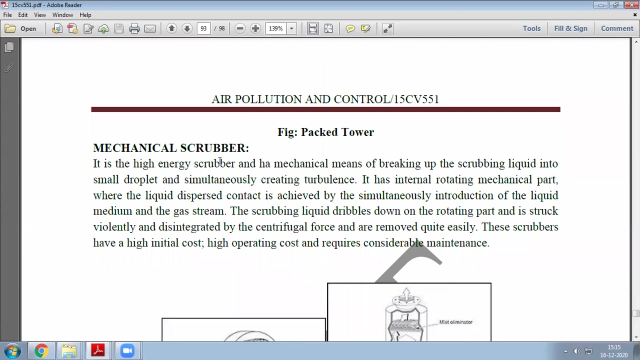 so that is here. uh, the centrifugal force are removed quite easily. these scrubbers have high initial cost. this all advantage is not that they're given high initial cost, high operating cost and require considerable maintenance. okay, so this is all you go through. advantage and disadvantage. okay, yes, 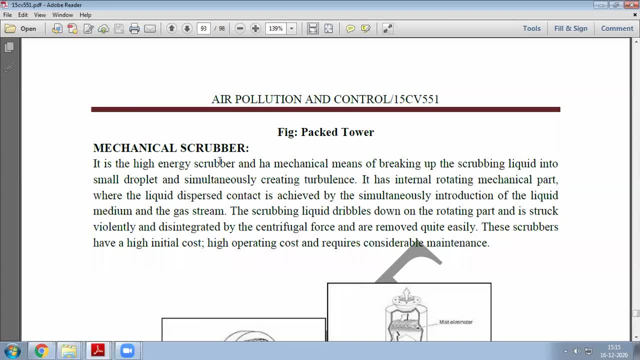 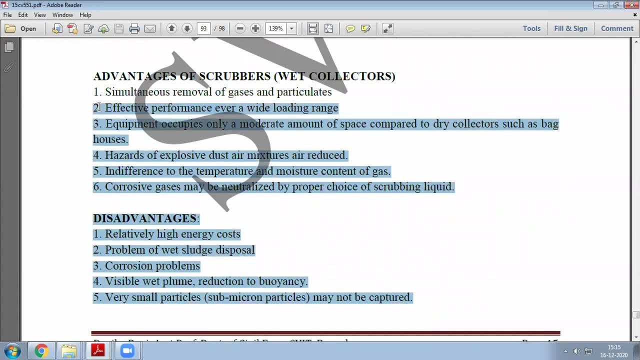 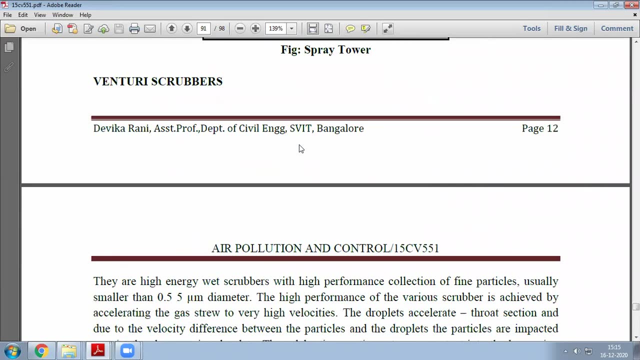 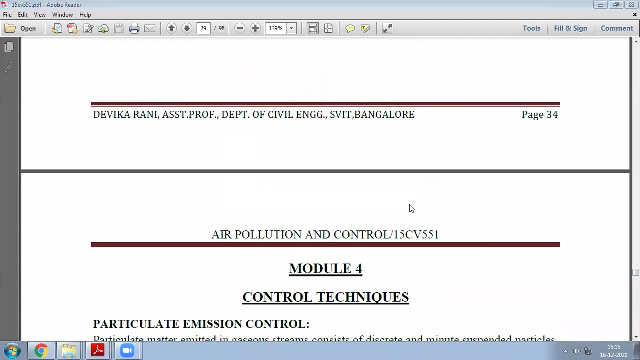 okay, then i think this fourth model i covered. this advantage is not that you go through this and i think any one question i will ask you to know- uh, any of the one here, and he this one also will ask. okay, last 10 minutes left for me. 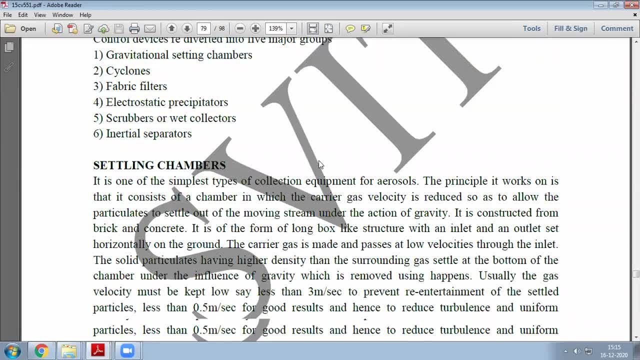 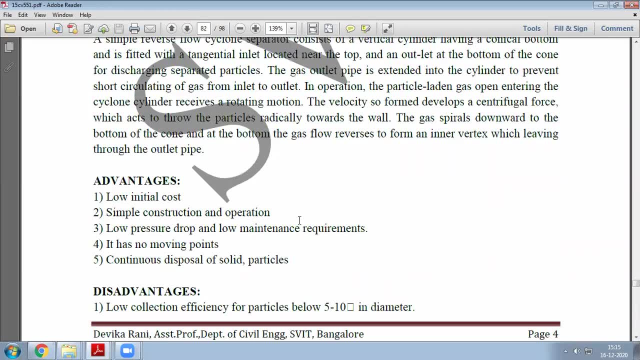 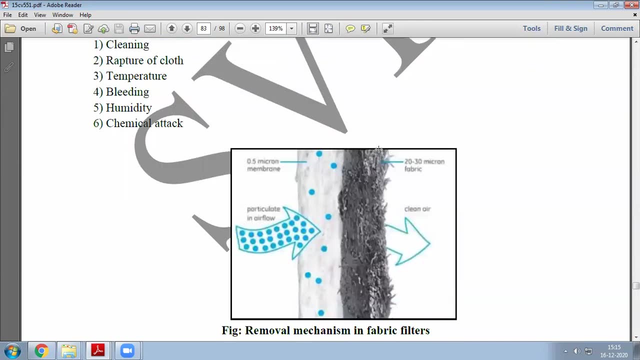 i think i covered most of the fourth model particulate matter. i covered cyclone and gravity separator. these two things i already covered in the last class. today i have done what the fabric filters means nothing but the fabric cloth material which was there. it was that i covered. next i 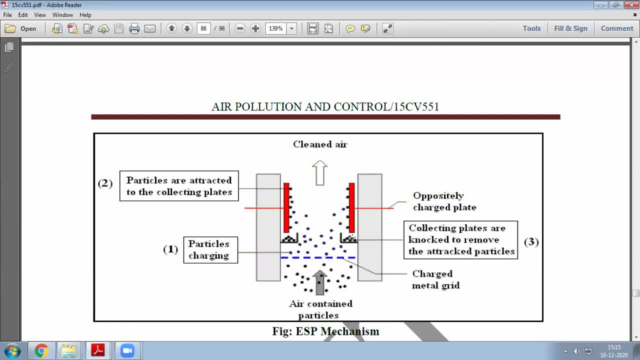 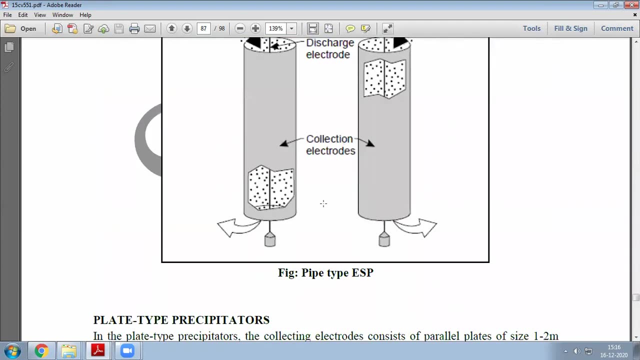 thought about what electrostatic precipitator- because of the potential difference, electrostatic- created this. electrodes made up of oppositely charged of the particulate which is entering because of this attraction, all particulars are collected here and clean air is going. this i covered and this how. what are the types? i think i covered plate type and pipe type. 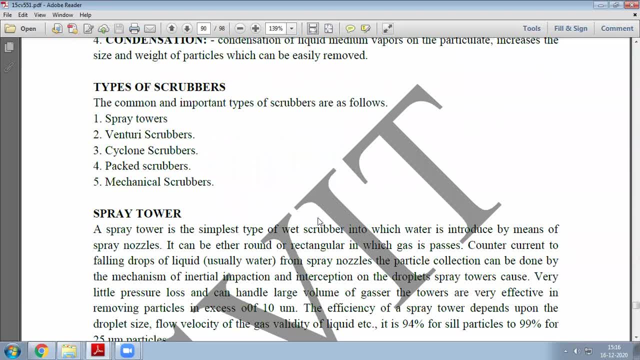 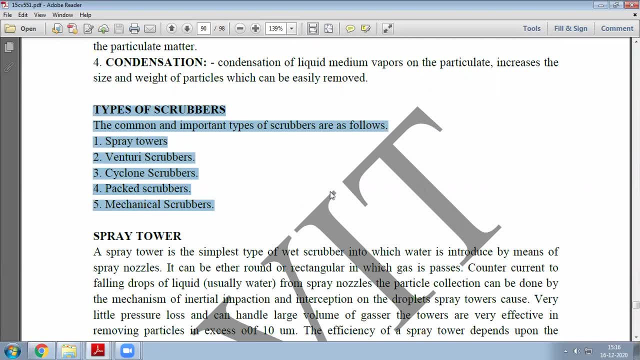 and after that what i covered, i thought about more on this scrubber- anyone scrubber, they might ask this. all five i think i covered, okay, so today up to that, this much, only tomorrow i try to do with model. okay, this is very lesser less to study this model, very easy, so go through. 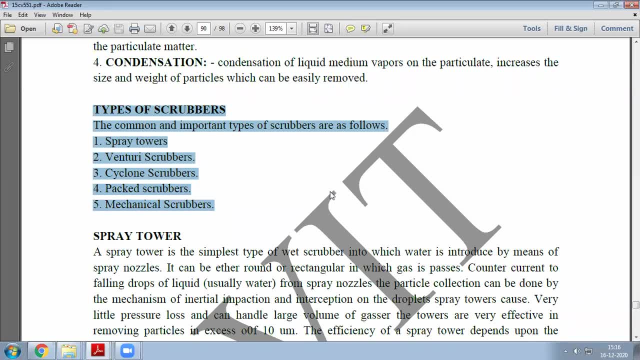 it. i think i will end the session, is it okay now? hello gonasri, are you there? okay, okay, okay, okay. hello raven, shakhi, shaheed and amrit: okay, yes, sir, okay, i will end the session. uh, you go through all this thing. okay, i will.